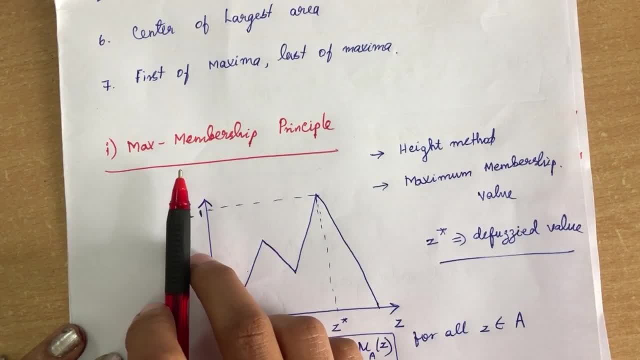 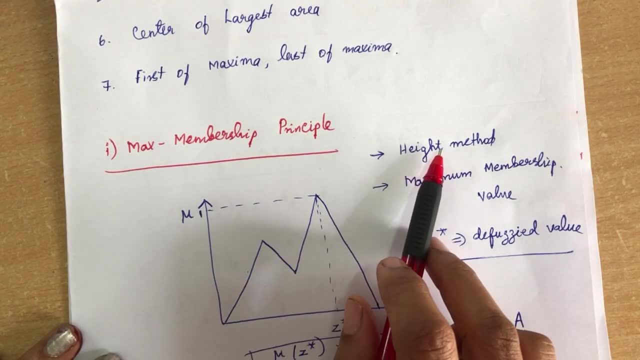 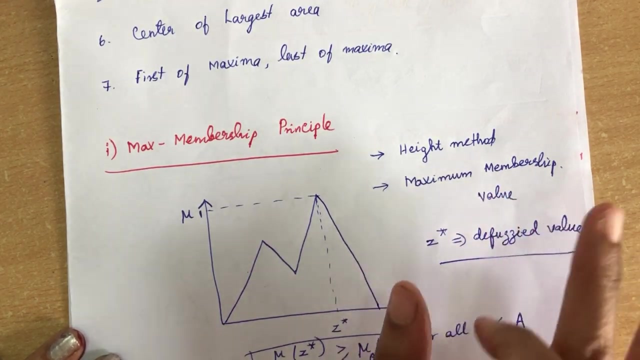 we will be discussing one by one. First we move on to the first method, that is, maximum membership principle. So this method is otherwise called as height method. This method will always give you gives you maximum membership value of a fussy set. So this method will give you maximum membership value of a fussy set. So this method will always give you maximum membership value of a fussy set. So this method will also give you maximum membership value of a fussy set, So this method will always give you maximum membership value of a fussy. 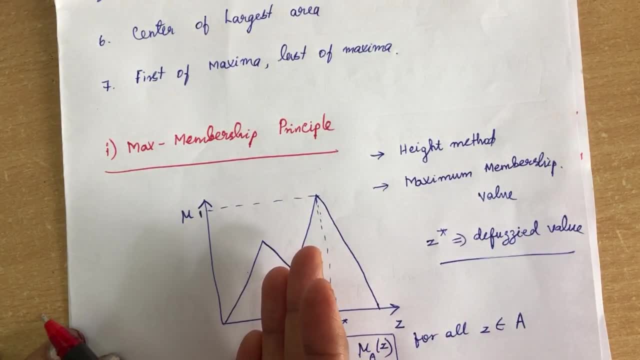 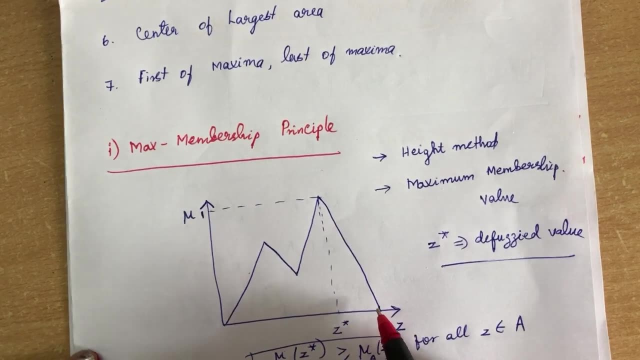 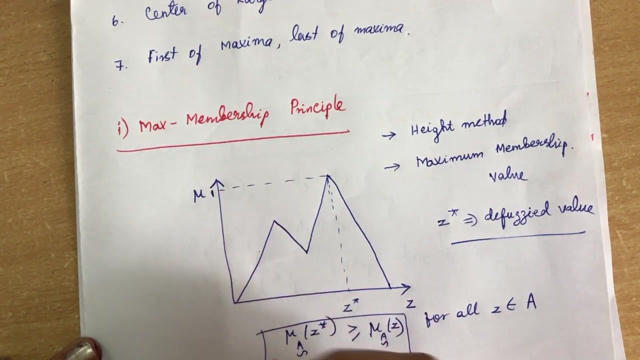 function Okay. So this diagram I have got by taking the union of two fussy set. So after taking the union of two fussy set, I am getting this diagram. So here in this diagram I have taken this Z as X axis and membership values in your Y axis. So by seeing this diagram, 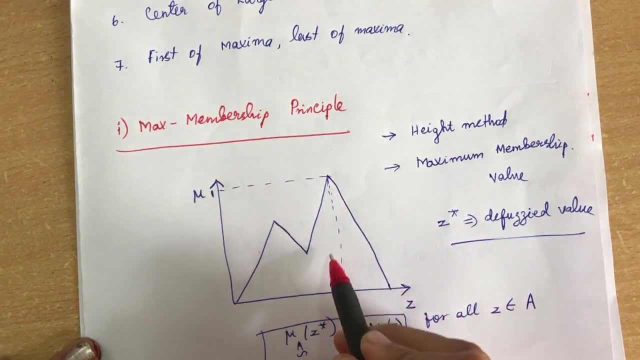 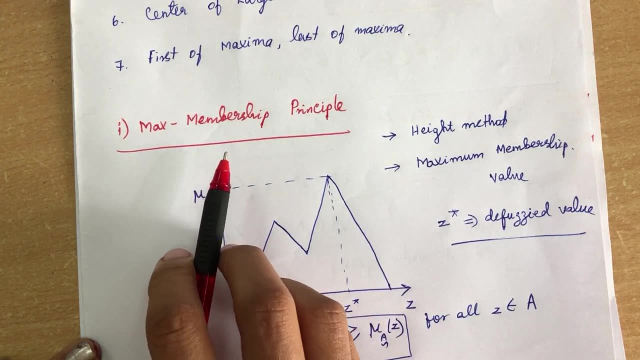 you can see that you can be. there is one point which is having the highest peak of all the values, That value which is reaching the value called one. So we are going to consider convert a fussy set into a crisp set. so for converting this we are going to use this. 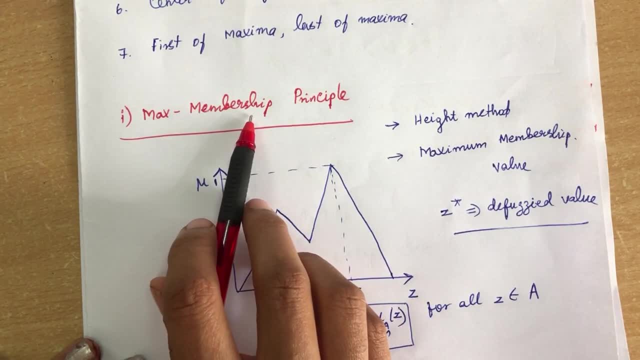 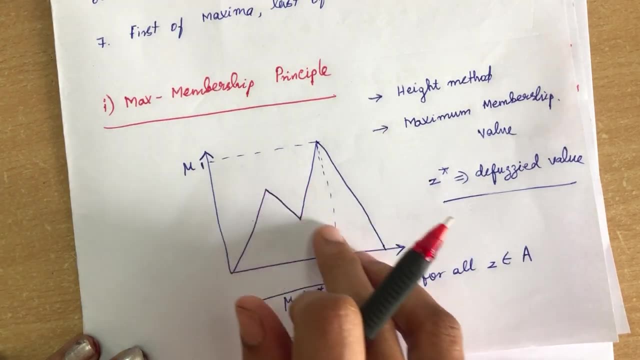 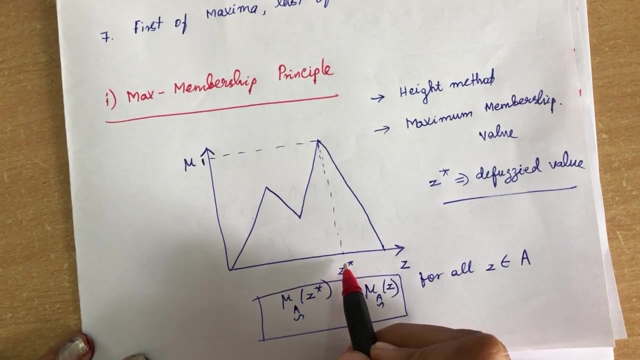 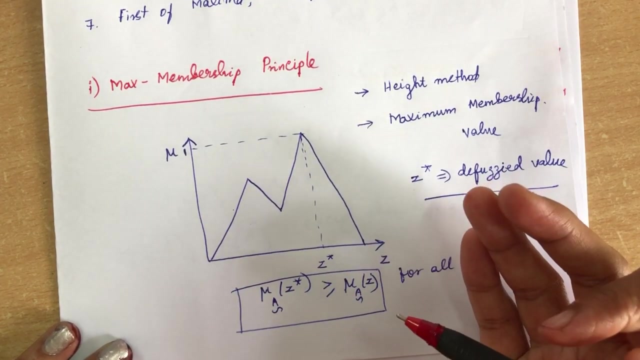 principle, maximum membership principle. so by the name itself it says that it will always get- takes the highest membership value. so which is having the highest membership value among all the values in this? so only this particular point. that means z bar is having your highest membership value. so this z bar is nothing but your d for c5 value. this value is your crisp value, so we can. 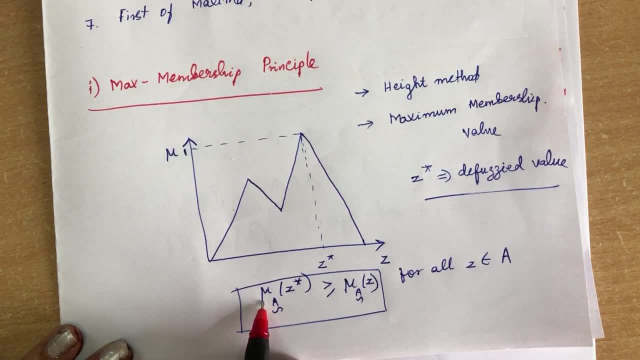 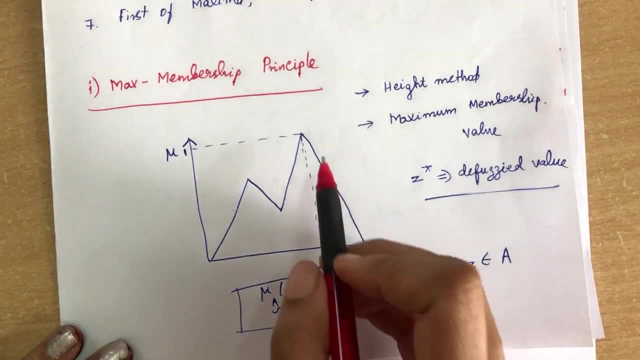 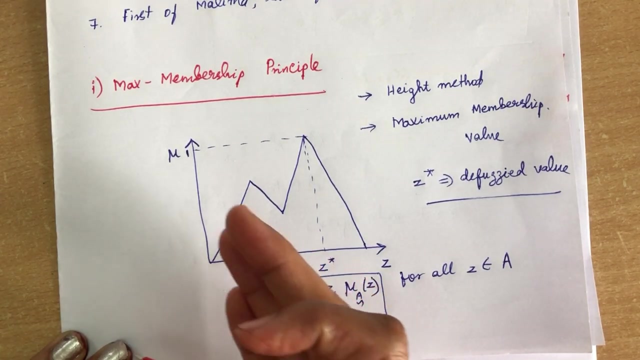 also say in a diagram, in an equation saying that membership value of z star is greater than or equal to membership value of other values. you can say that membership value of this z star is greater than or equal to. it may be greater than or equal to the membership values of other values. 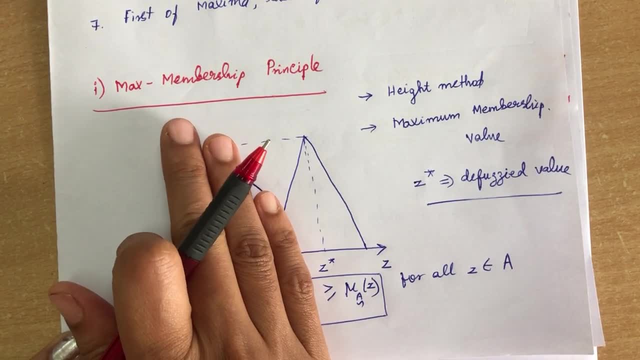 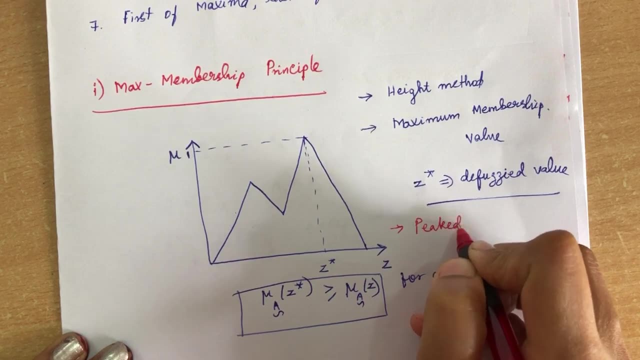 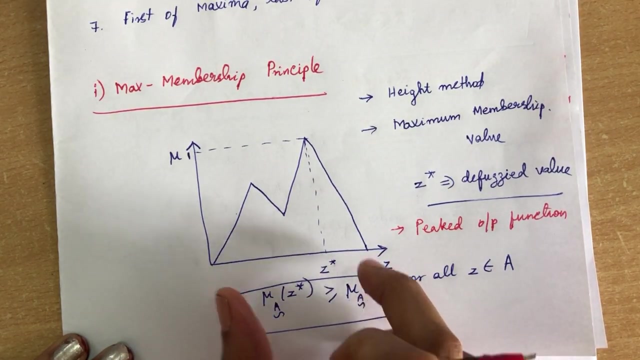 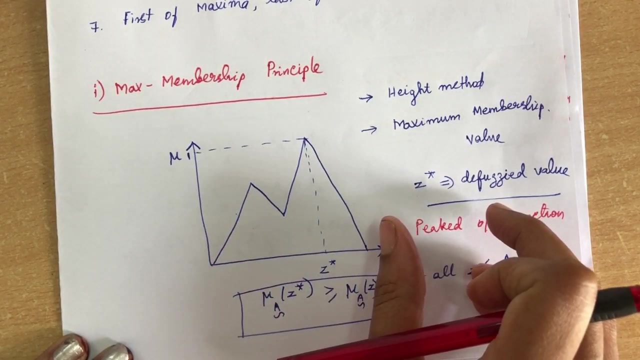 that is the equation for your math membership principle. but this particular principle can be used, can be applicable only to peaked output function. so so in this diagram, this particular diagram, it is having a peaked output function, so this particular principle will be applicable only the to these types of functions. so, where you can able to apply this particular principle and you can find out, 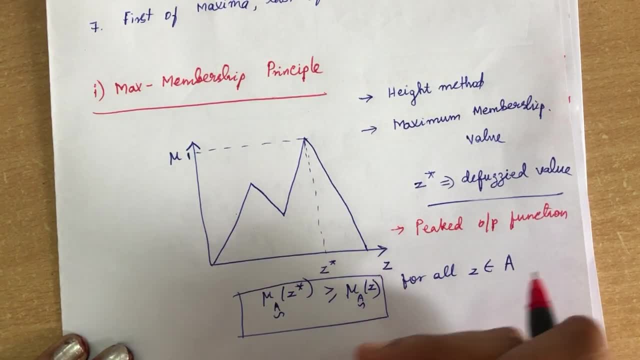 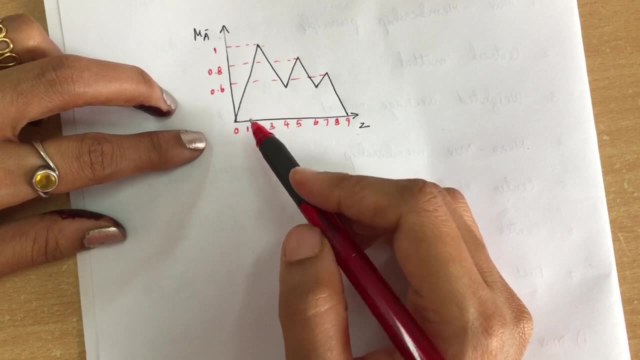 you can able to convert a fussy value into the. that is like crisp value. okay, let's see one example. so let's say we have a fussy set of z bar is greater than or equal to z star is greater than example. now let me explain one simple example for this maximum membership principle. so here i have. 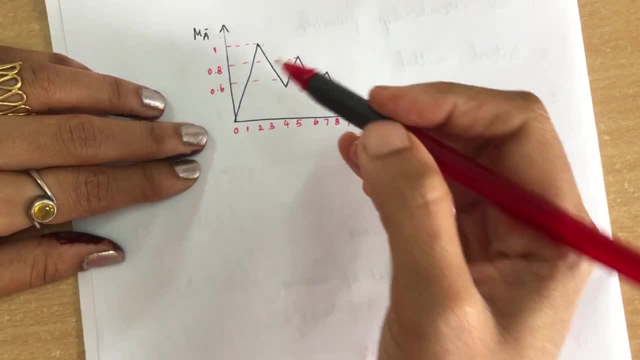 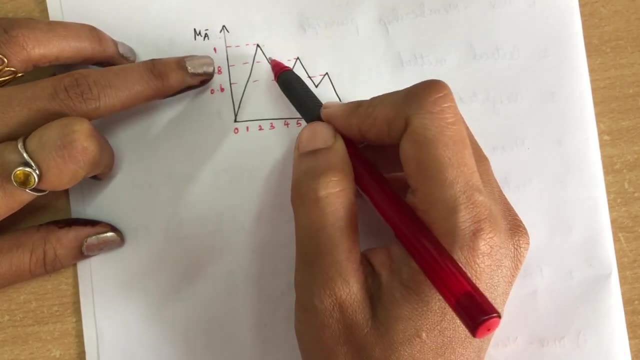 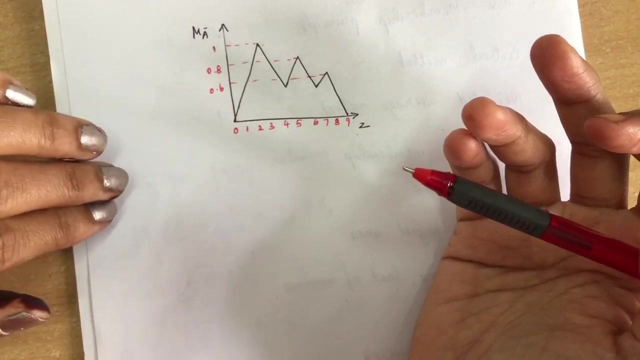 considered this diagram where x axis, i'm taking z values, in y axis i'm taking all the membership values. so this particular function is: this is got by the taking the union of three fussy sets. okay, so now i want to convert this fussy value into a crisp value, so by using maximum membership. 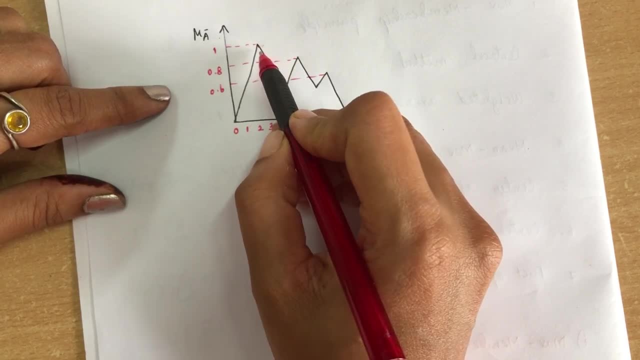 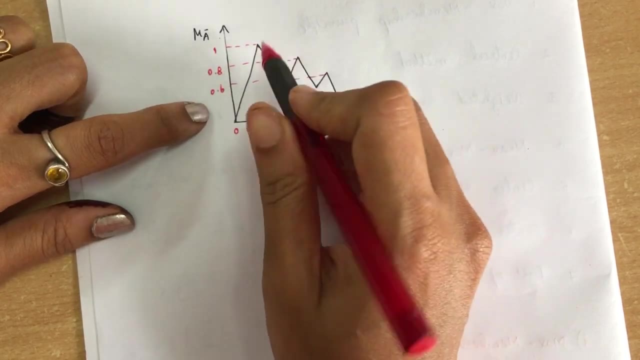 principle. so here i can see that there is one particular function that is greater than or equal to z star in particular point where it is having the maximum membership value, that is one, and this point is having 0.8 and 0.6. so this particular point is having only the highest peak value. so 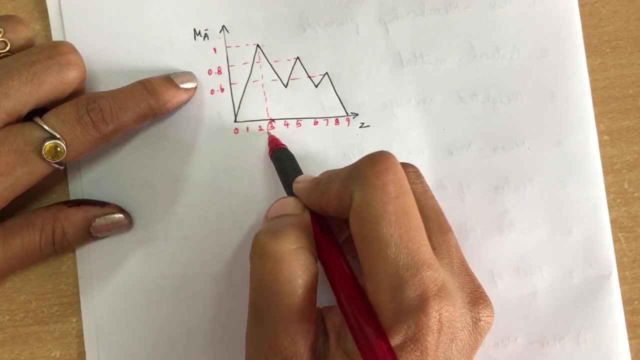 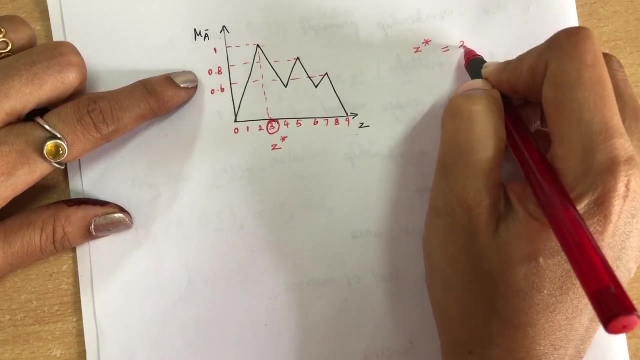 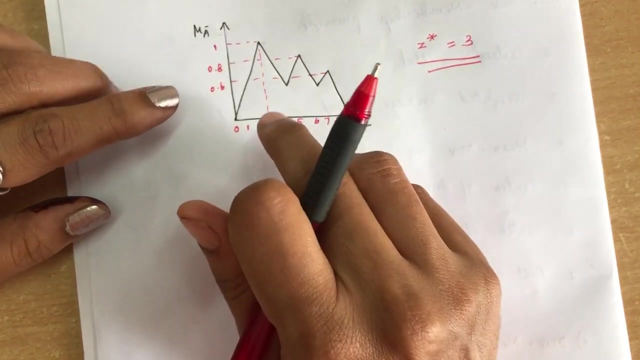 i'll extend this point down. so this particular value is called your z star. so now z star will be will be equal to 3, so this is your crisp value. this is your defussified value. this is how you will convert a fussy value into a crisp value, so this particular function is called your z star. 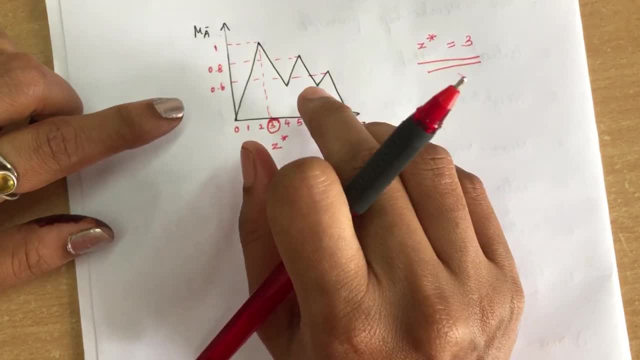 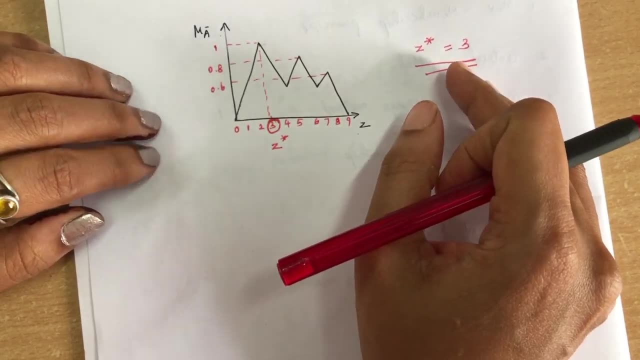 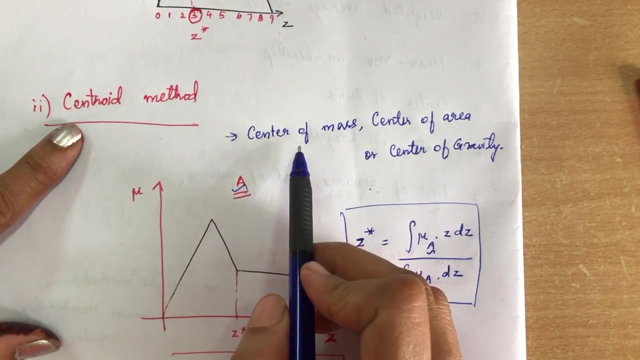 into a crisp value using maximum membership principle. so any example is given for you. it is very easier: by using maximum membership principle, you can convert into a defussified value. okay, so moving on to the second defussification method, that is, centroid method. this method is otherwise called center of mass or center of area or center of gravity. 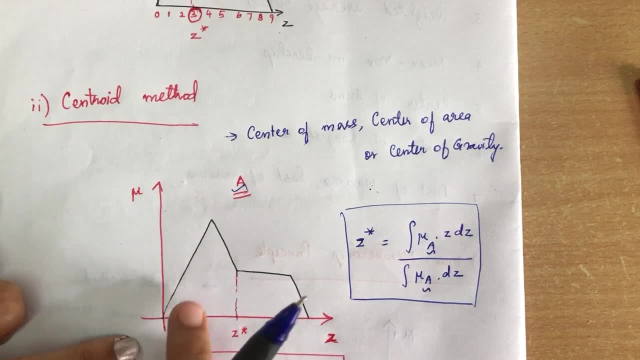 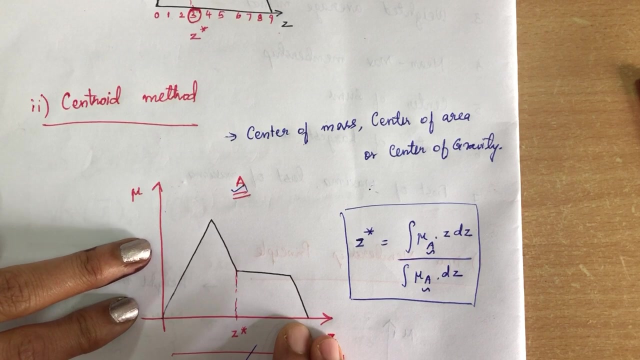 so here i have drawn one diagram where i have got this particular diagram by taking the union of two fussy set. okay, so in this diagram, x axis, i am taking z values, in y axis i am taking the membership values. so for this particular fussy set i need to find out the defussified value. 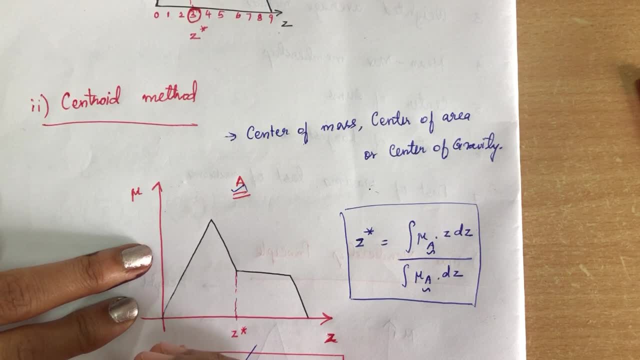 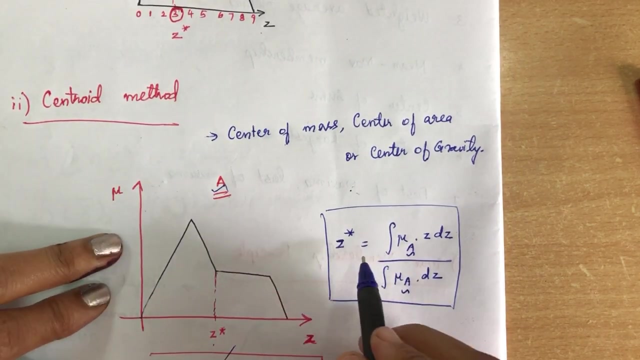 so this defussified value is received by taking the centroid between the two fussy set, the centroid value. it will be got somewhere in between, like this, between the two fussy set. let me call it as z star. so we can write an equation for the centroid value. so we can write an equation for the centroid value. 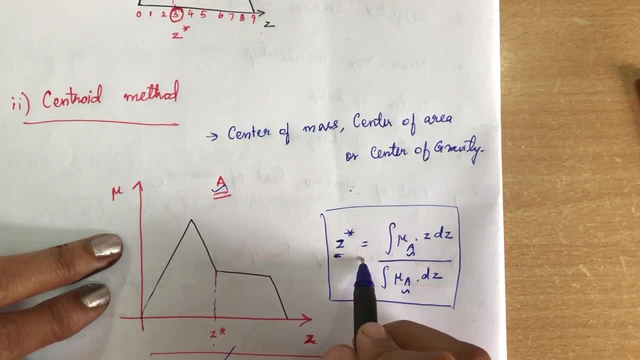 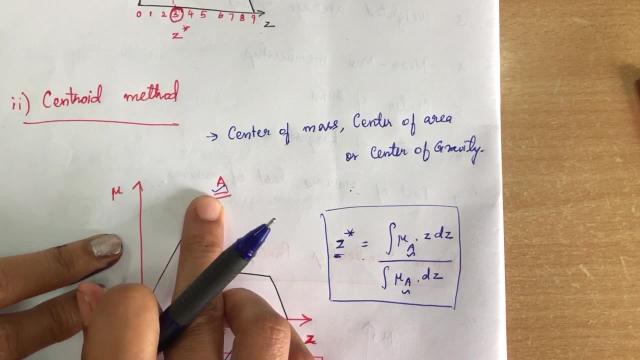 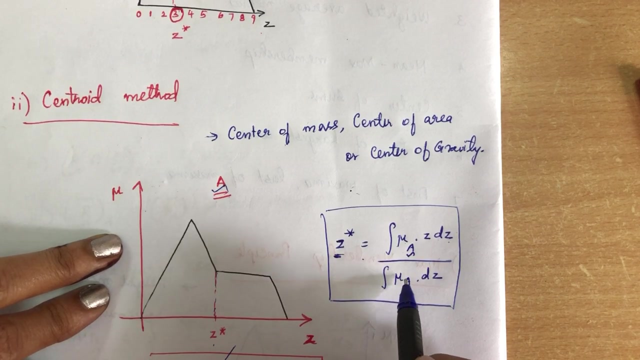 this defussified value, z star, is given by taking an algebraic integration of membership value of a. this is the fussy set named as a. so a into z is dz divided by integration, algebraic integration of membership value of dz. okay, by using this equation we can find out the defussified value. 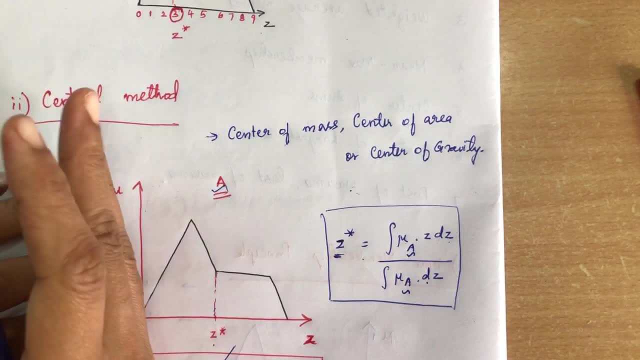 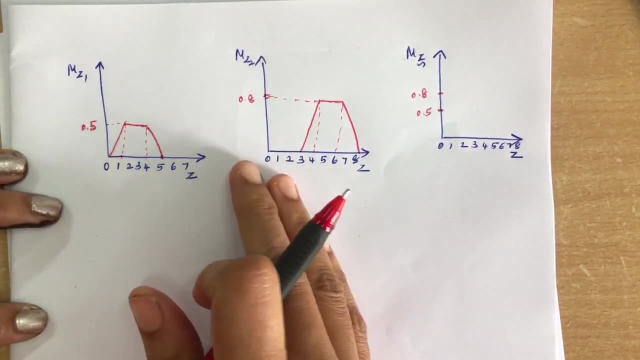 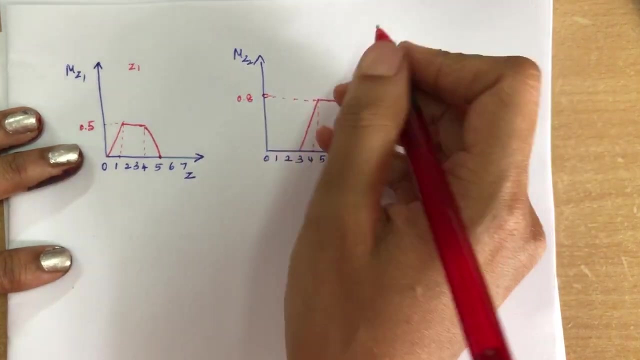 let's explain with a simple example. okay, so the centroid method. you will be using this formula and you will be finding out the defussified value. so i have drawn three diagrams. so here the first fussy set. let me call this fussy set as z one. the second fussy set i am calling to be 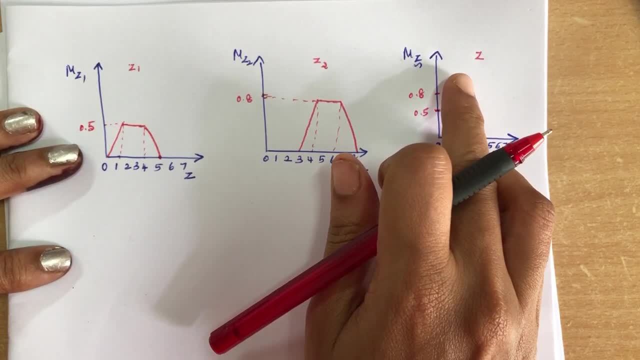 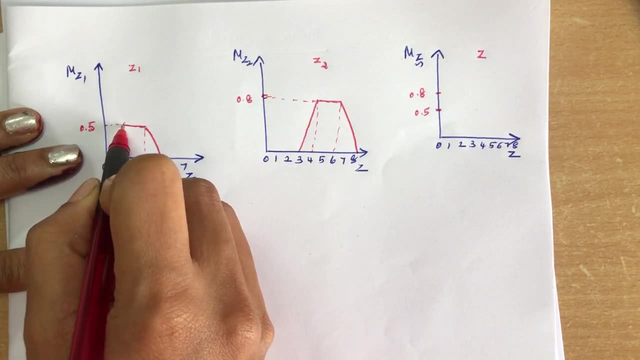 z two. so this the z it will be. this it is. it is got by taking the union of two fussy set. first the fussy set, it starts from zero and it it is having a straight line from one to four and then it is coming downwards and it is ending at five. 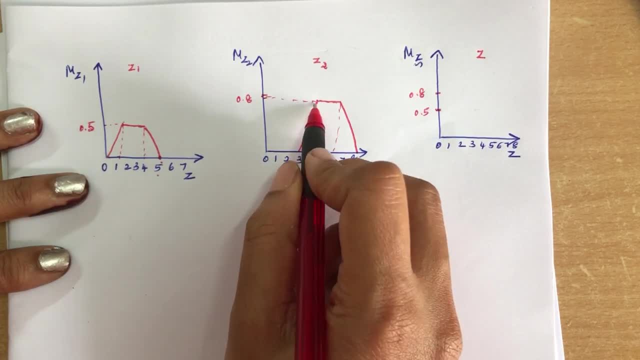 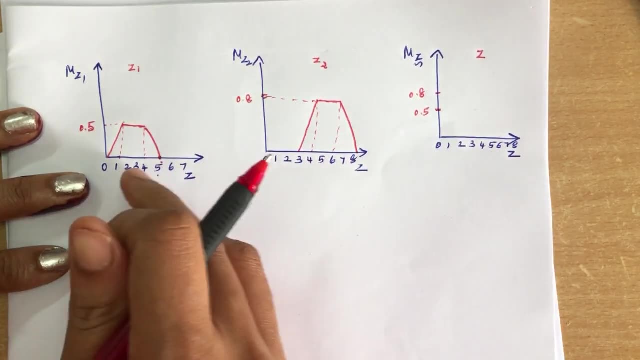 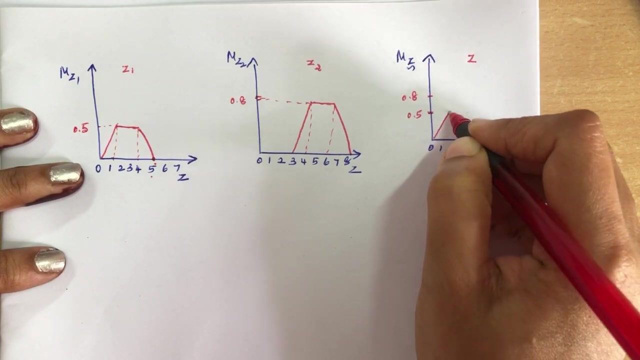 coming to this z two, it starts from three and it is reaching four to its peak, and then six, and then from six onwards it is going down. so by taking the union of two fussy set, it is some, simply by adding the two fussy set. so first it starts from here and then 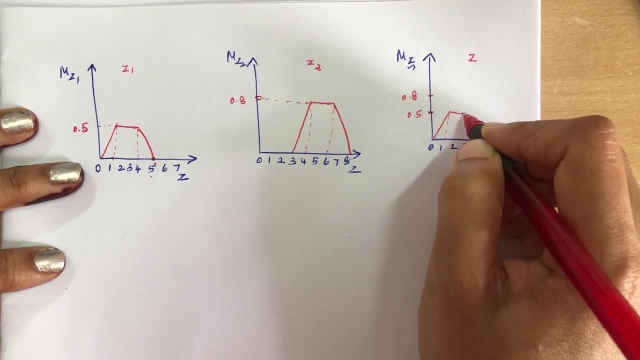 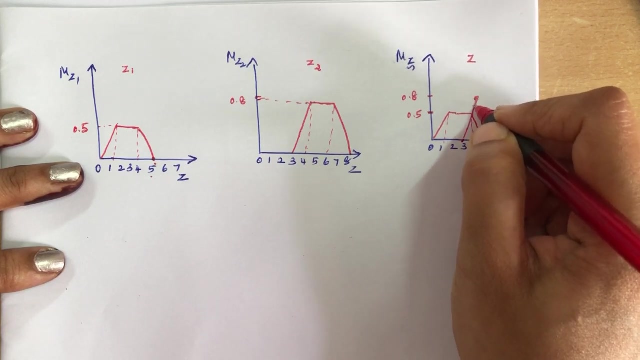 it goes till. so one goes till three, four, right, okay. and then it is ending here and we will draw the second diagram also over here. so it is starting from three and it is having a membership value called eight. okay it is, it is reaching a peak at this region. four: 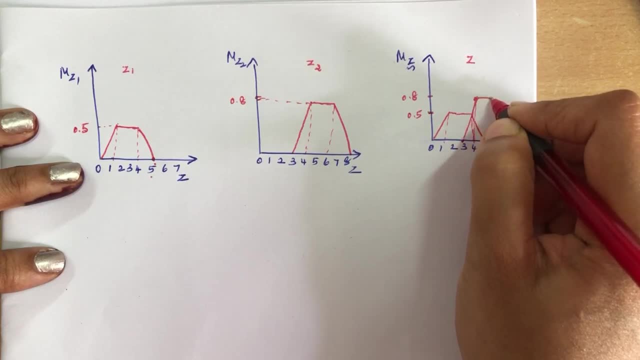 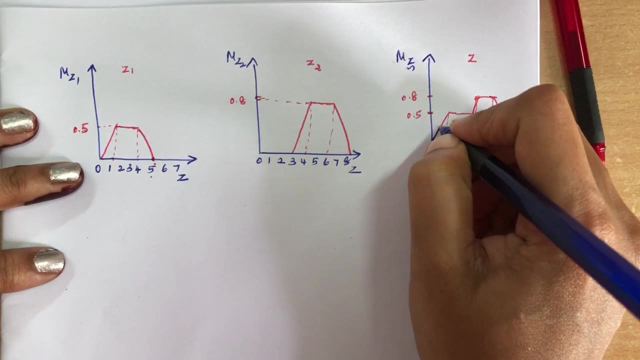 and then it goes till six, and it is coming to eight. okay, so this is what you will get for your: the union of two fussy set. okay, this is how you have it. How to make a fussy set. How to make a fussy set. 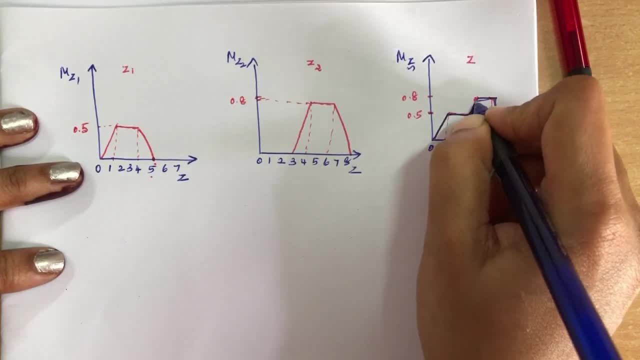 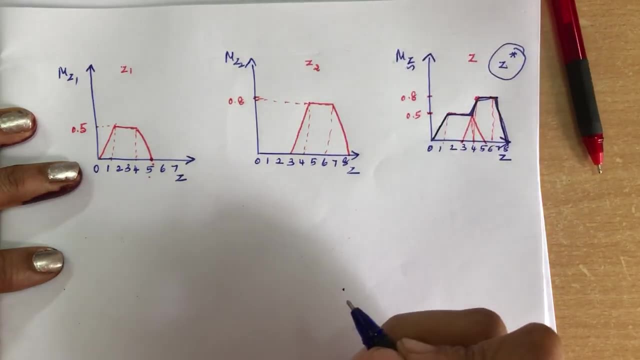 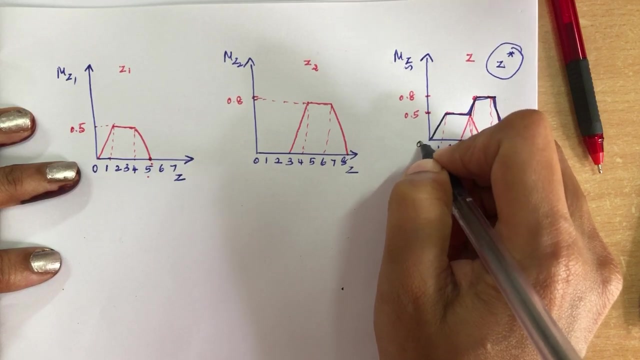 After this, you need to find out, you have to find out, the union of two fussy set. so now, for this particular fussy set, you need to find out z-star diffusified value. so for finding out the defusified value, i am going to split into so many parts, okay, so i am going to name. 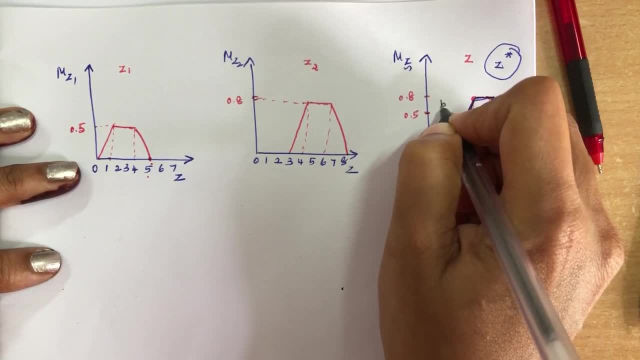 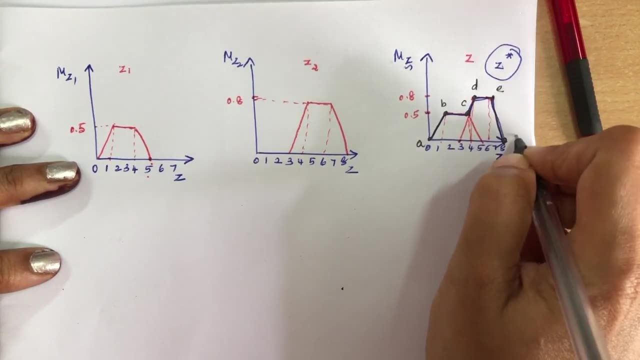 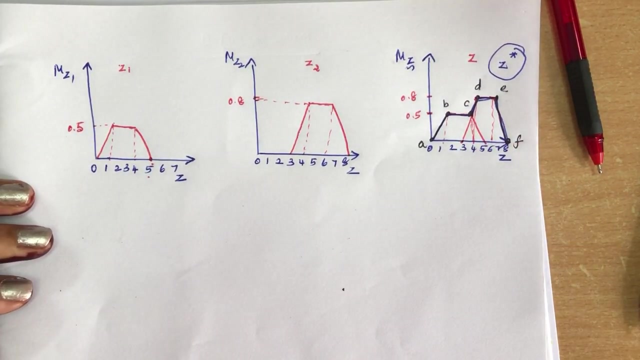 this particular point as A and this particular point im naming to be B, here im naming to be C. this point is D, over here it is E and then here it is F. So I am going to use integration method for this and I am going to find out the de-fuscified value. 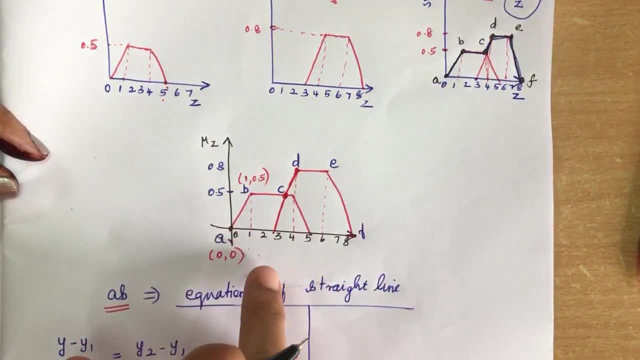 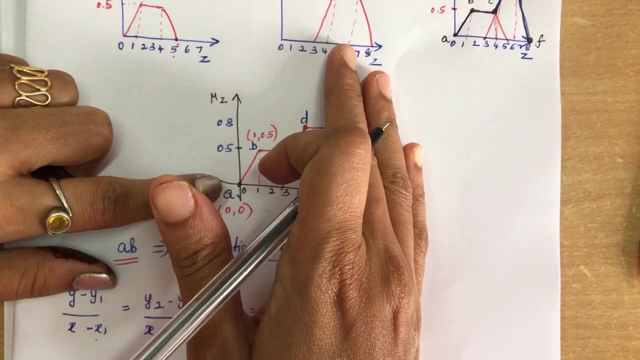 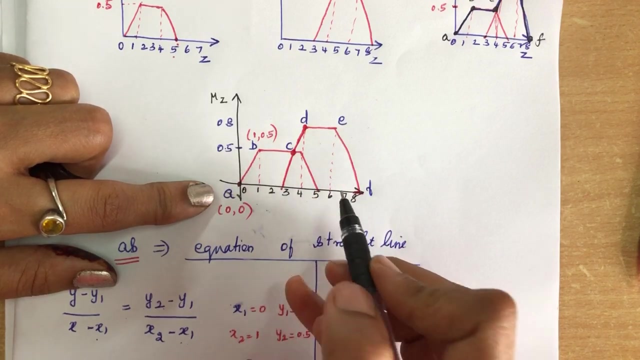 okay. So I have taken this diagram and redrawn this diagram over here. So here I have. this particular diagram is got by taking the union of two fussy set, So I am considering all these points as A and this point is B, C, D, E, F. So I am going to use centroid method to find out the 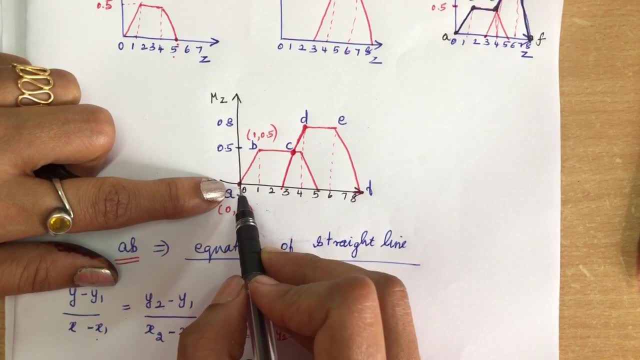 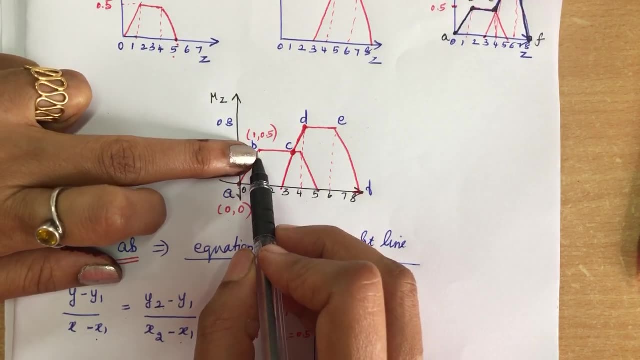 de-fuscified value, So let this point be A. So what is xy value? xy value is 0, 0, okay, So first I am taking this AB pointer and B point. what is xy value? x value is 1 and y value is 0.5.. So 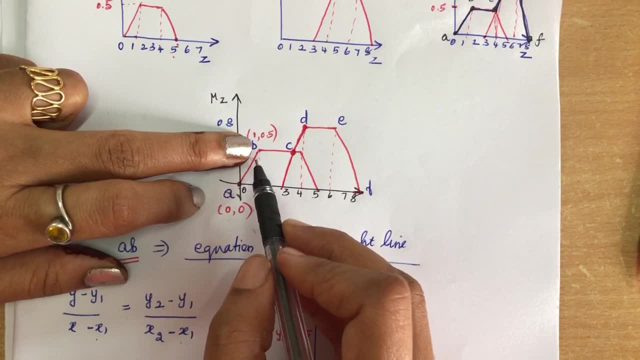 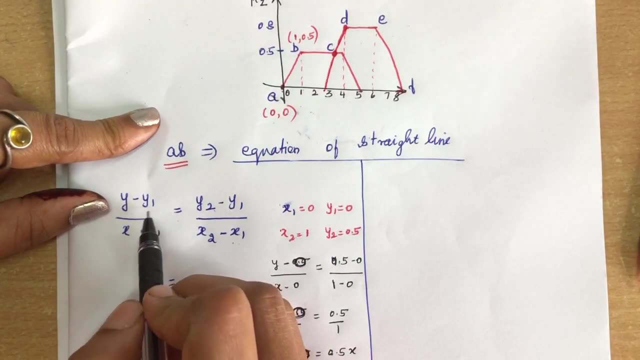 it is 1, 0.5.. So I am going to use the equation for the straight line. What is the equation for the straight line between A B? So it is nothing but y minus y1 divided by x minus x1, that will be. 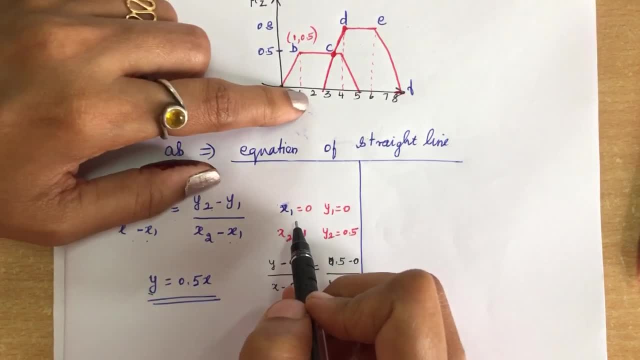 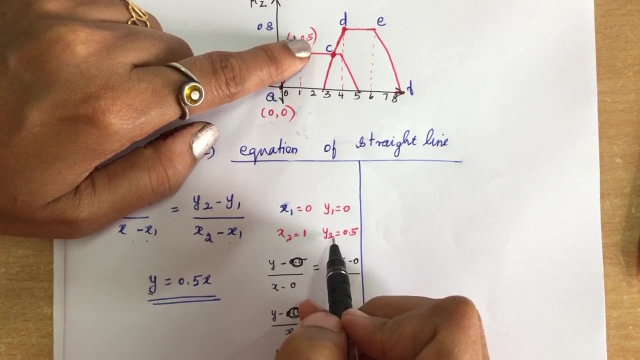 equal to y2 minus y2.. So what is x1, y1?? x1, y1 is 0, 0.. What is x2, y2?? It is 1, 0.5,. okay, So now I will substitute. 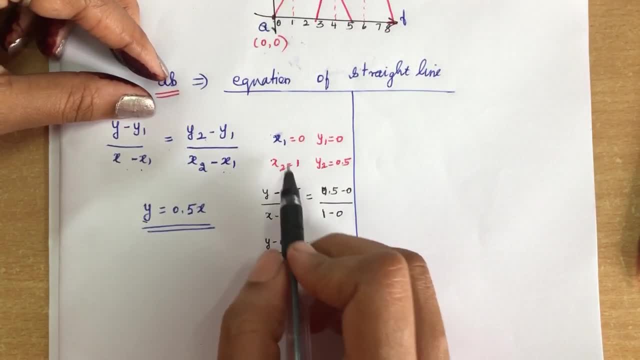 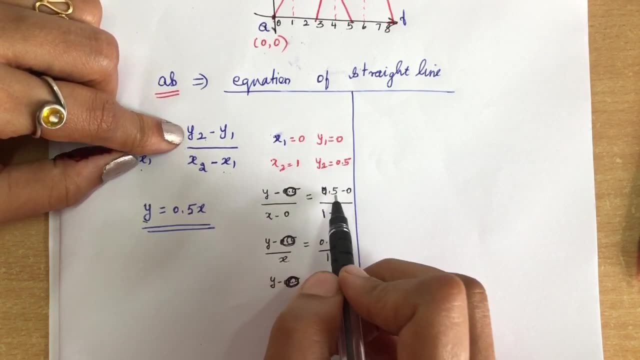 all these values here. So what I will get, I will get: y minus y1 is 0. divided by x minus x1 is 0, that will be equal to y2.. y2 is 0.5 minus y1 is 0. divided by x2 is 1,. 1 minus x1 is 0. So I will get: 0.5 minus 0 is 0.5.. So I will get: 0.5 minus 0 is 0.5.. So I will get: 0.5 minus 0 is 0.5.. 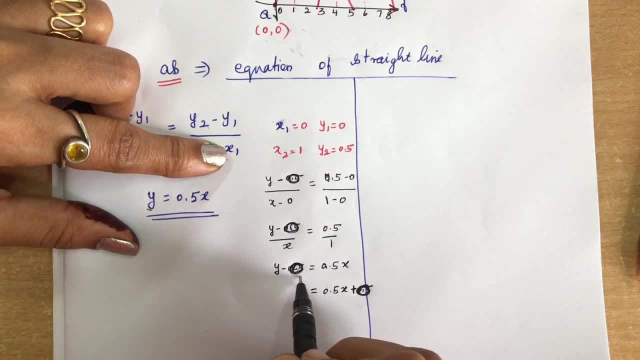 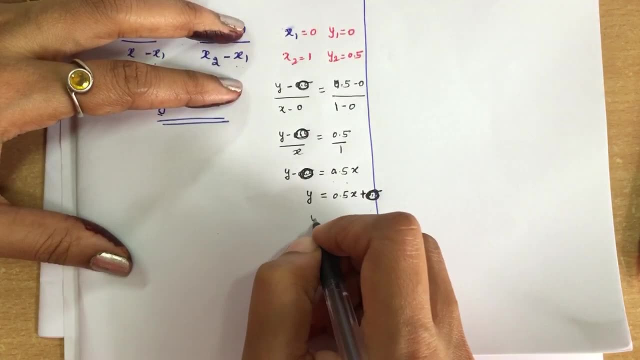 And this is 1, y minus 0 divided by x, that is y minus 0 will be- I am taking cross. multiply y minus 0 will be 0.5 into x, that is y will be equal to 0.5x. Okay, this is what I have written. 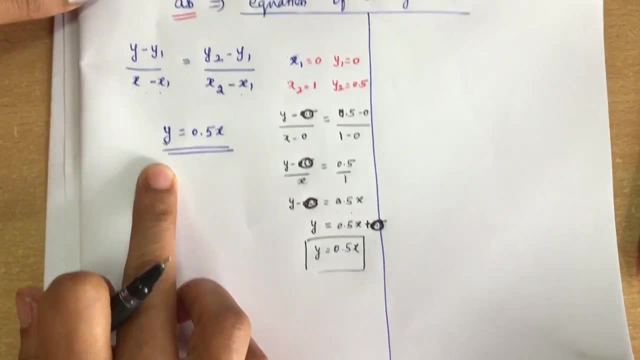 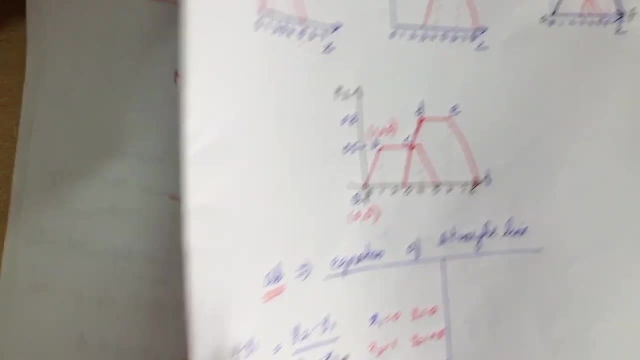 here y equal to 0.5x. okay, So the limits will be between 0 to 1.. You can see the integral limits. So the formula for this particular method is like this: The formula is taking a centroid. 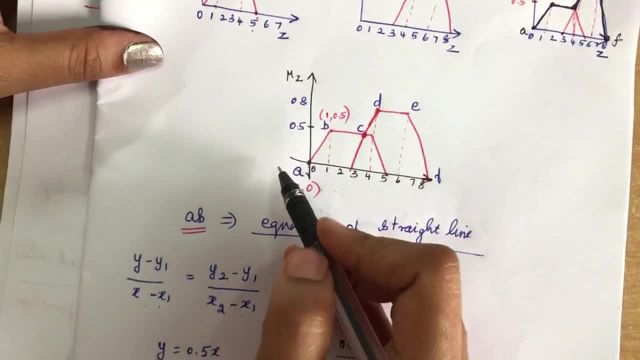 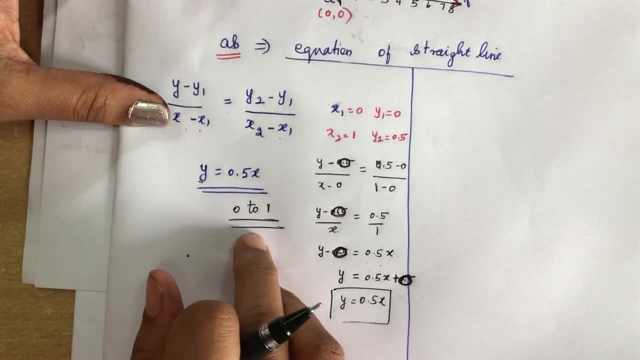 taking the integration. So what is the integral limit Between? it is from the straight line, 0 to 1.. So I will write: the integral value will be 0 to 1.. Likewise, I will be finding out the equation for BC, equation for CD, DE and EF. okay, 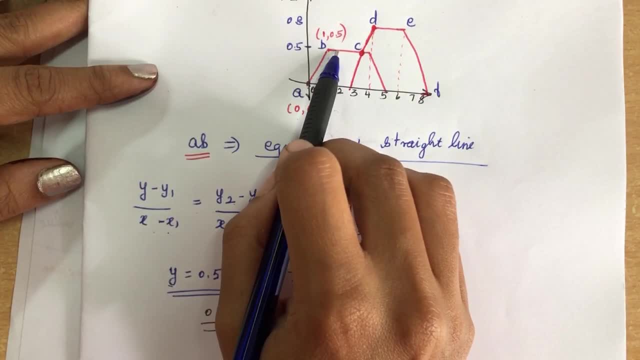 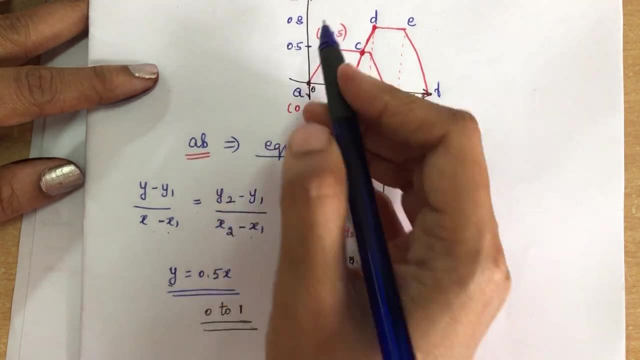 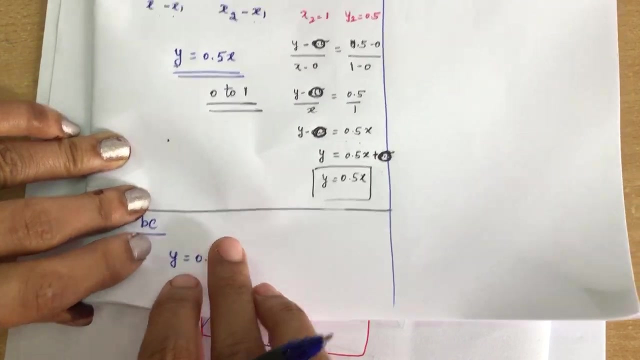 Second, we will find out the equation for BC. Since this particular line is parallel to this x-axis, then the y value will be equal to 0.5. It is having a value called 0.5. So the BC equation will be y equal to 0.5.. So, for the interval, if you take this, 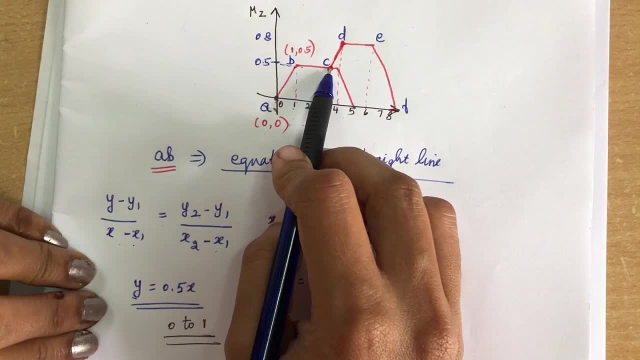 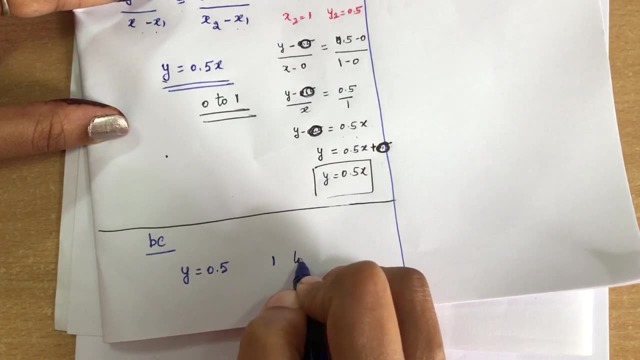 it is starting from the region 1 and it is ending at C. C will be somewhere in between 3 to 4.. So the integral value will be 1 to that is 1 to 3.5,. okay, Integral value is 1 to 3.5.. So 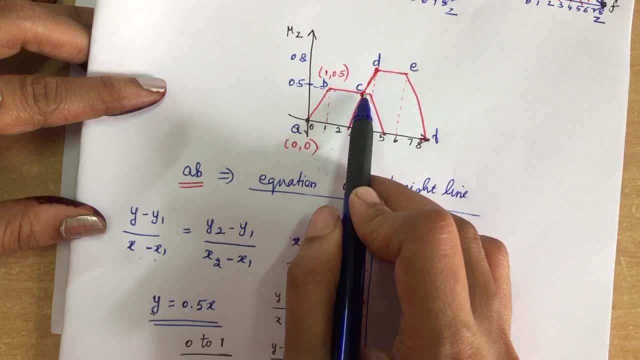 we are not considering 1 to 4.. Since it is ending over here, C point, we are having it between 3 and 4.. So we are not considering 1 to 4.. Since it is ending over here, C point, we are having it between 3 and 4.. 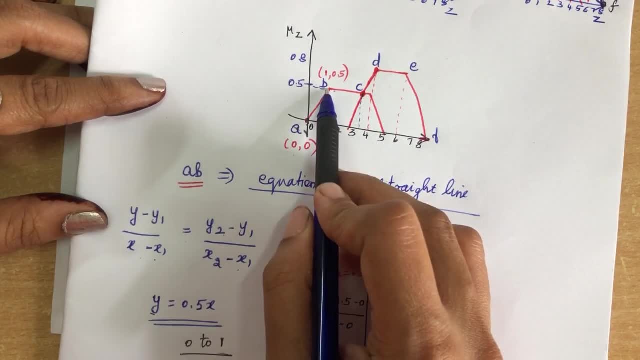 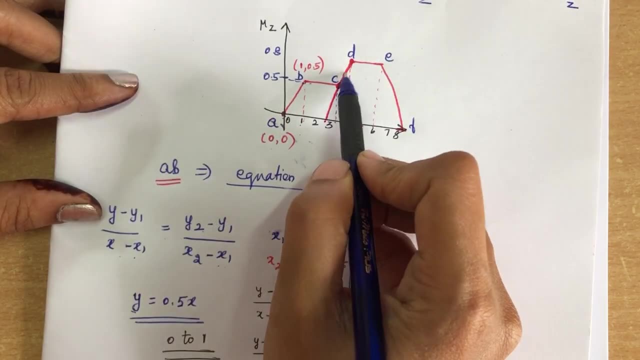 We are taking the value, integral value between 1.. It is starting from B, It is starting from 1.. It is ending at 3.5,. okay, This is the integral value. okay, Now we will find out the equation. 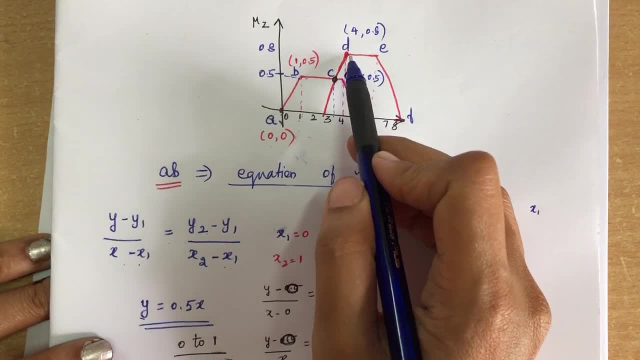 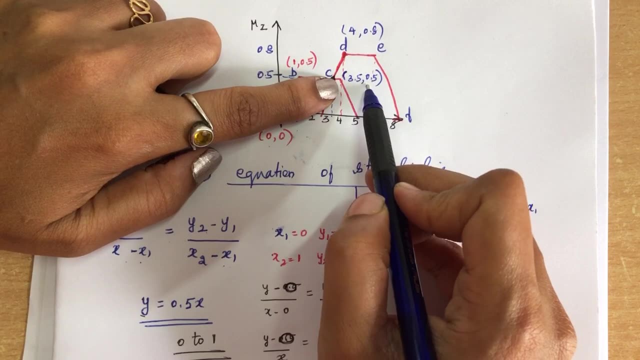 for CD. Now we will take the equation: CD, So CD. it is the point. This is point is 3.5 x and y value is 0.5.. So 3.5 comma 0.5 and this particular D point it is having x value 4. 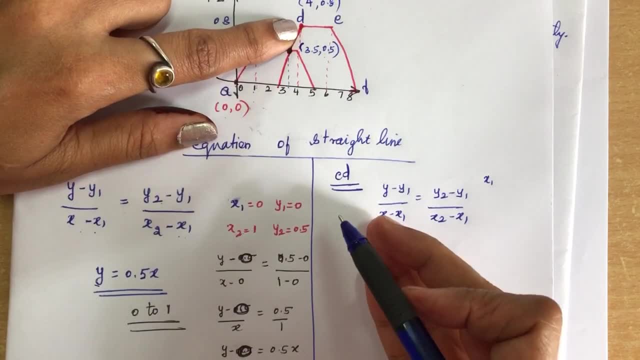 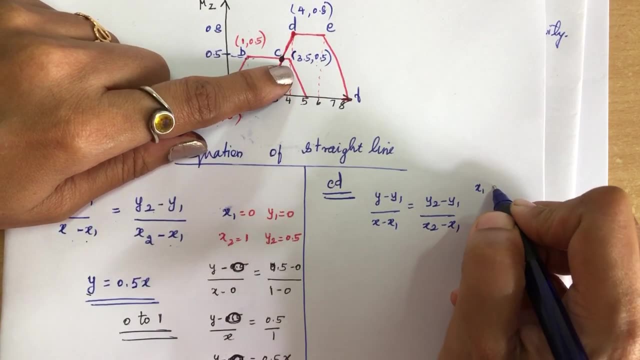 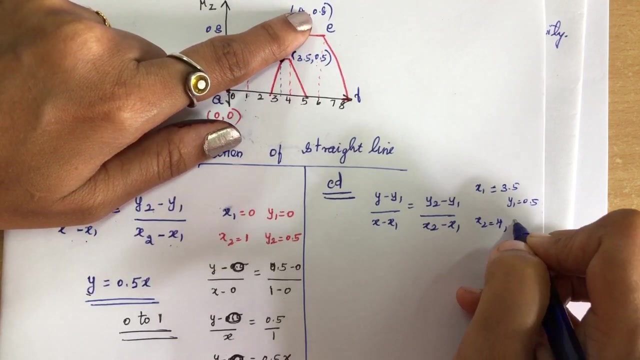 and y value 0.8,. okay. So we will use the same equation for finding out x1, for finding out the equation for that particular line. So here x1 will be 3.5 and y1 is 0.5, x2 is point, x2 is 4 and y2 is 0.8, okay. So when you substitute all these values, 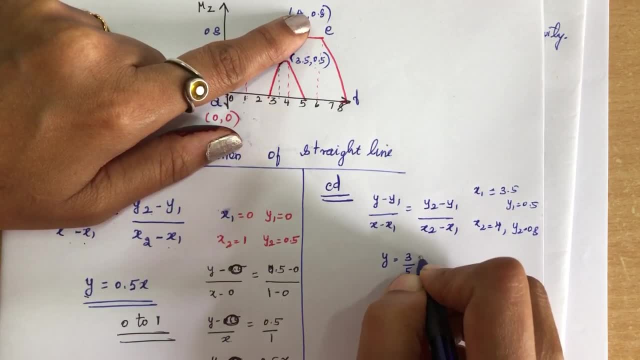 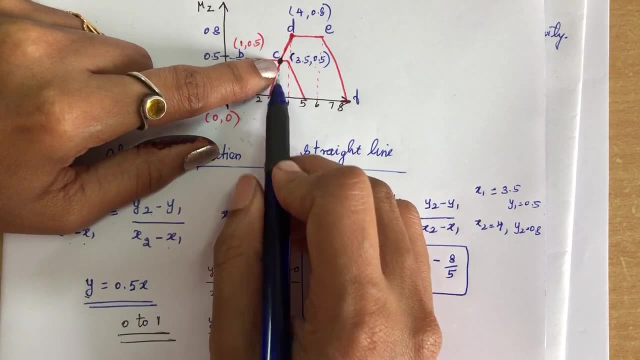 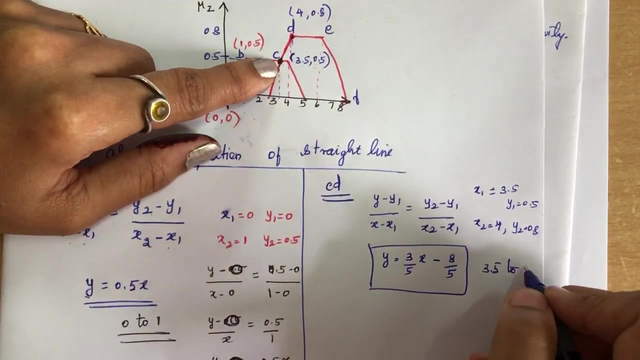 here you will get: y will be 3 by 5, x minus 8 by 5,. okay, And what is the integral value? Integral value, it will be between starting from 3.5.. 3.5, and it is ending at this particular point. It is ending at 4,. okay, So this is the equation. 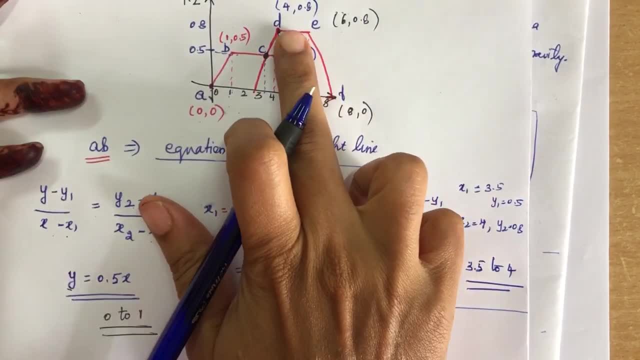 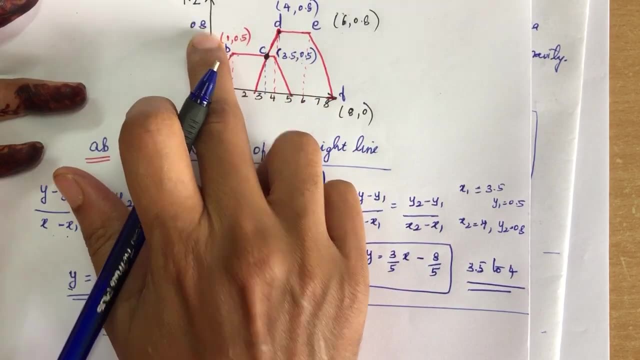 for this particular line, CD. So, coming to this point, DE. So DE is parallel to this particular x axis. So we will get y will be equal to 0.8.. So the equation for DE is y equal to 0.8. 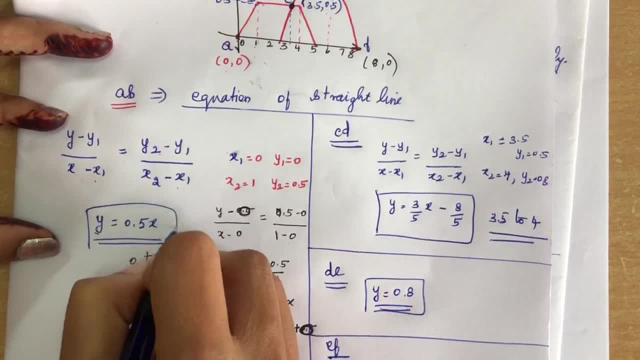 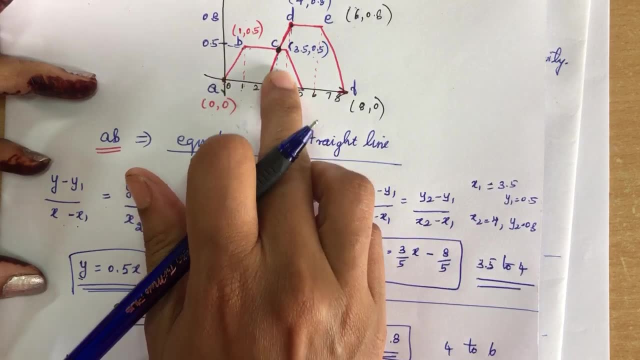 and the integral value will be between: So it is starting from 4 and ending at 6,, 4 to 6.. Okay, Starting from 4 and E ends at 6.. So I am writing 4 to 6.. Now we will find out the last. 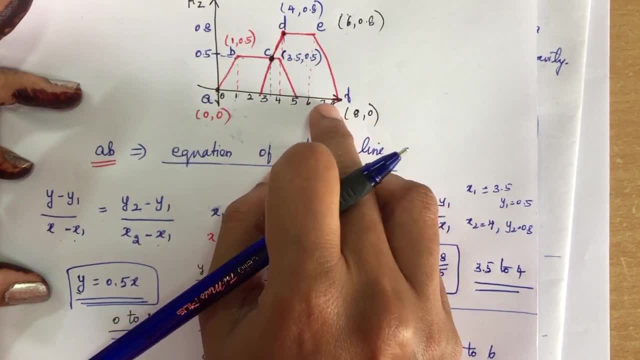 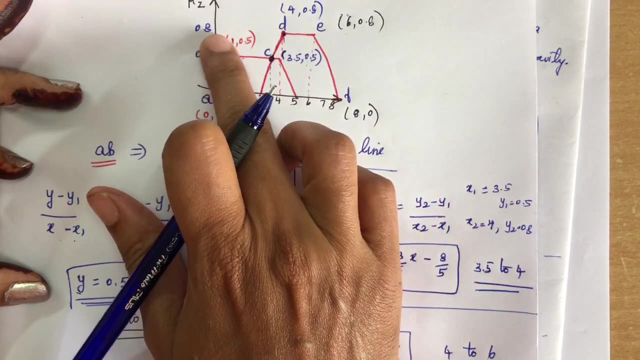 straight line. So it is from E to F. So what are all the points? It is, since it is 8 comma 0 over here and this one is 6.. So it is here. this point is 6, x value and y value is 0.8.. So we will. 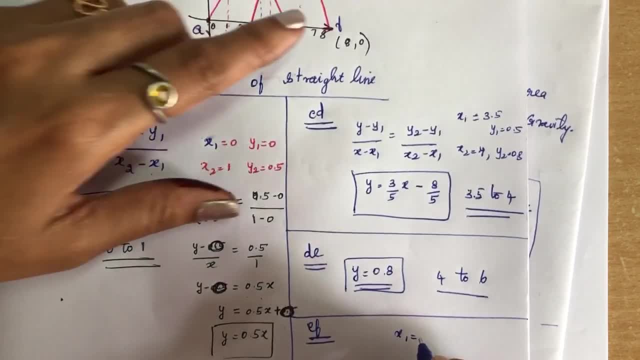 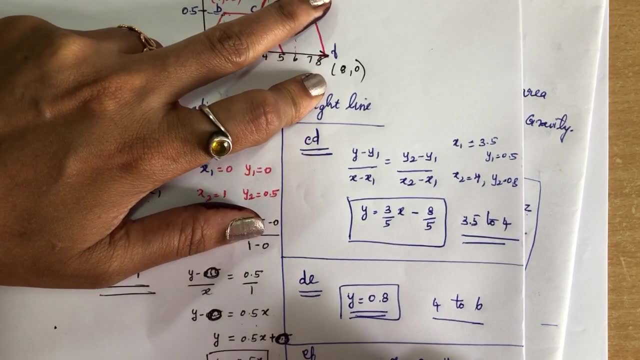 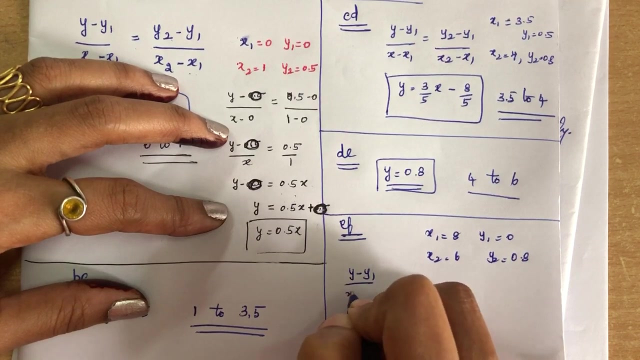 substitute these values over here. So x1 will be 8, comma, x1 is 8, y1 is 0 and x2 will be 6 and y2 is 0.8.. So substitute all these values in the equation y minus y1 divided by x minus x1. 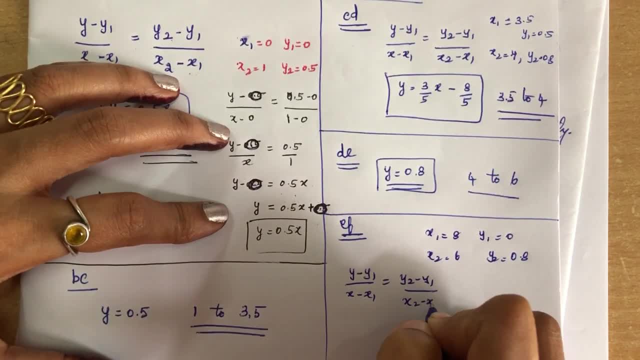 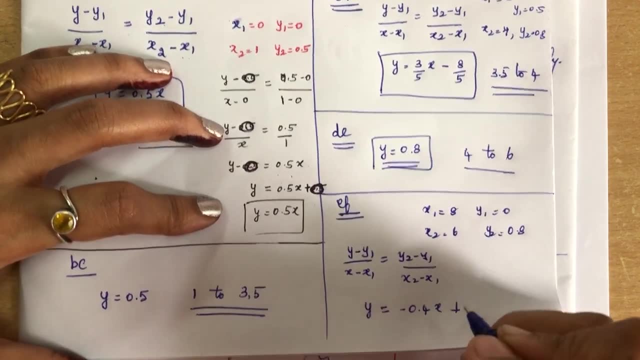 will be equal to y2 minus y1 divided by x2 minus x1.. So when you substitute this value, I am getting y will be 0.4x plus 3.2.. Okay, This is what I am getting, this. So what is the? 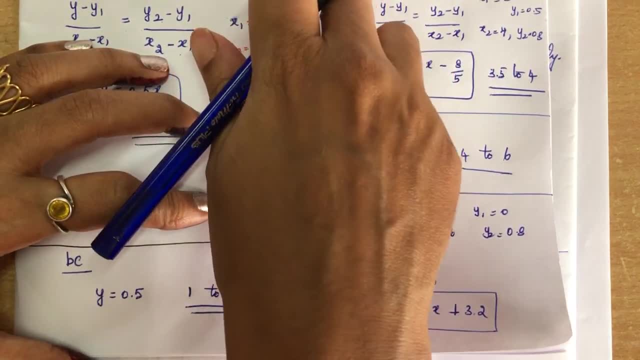 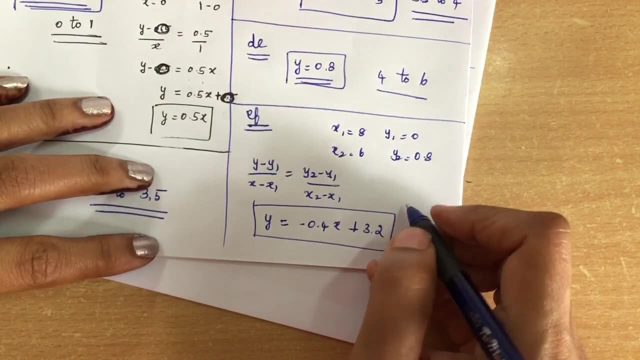 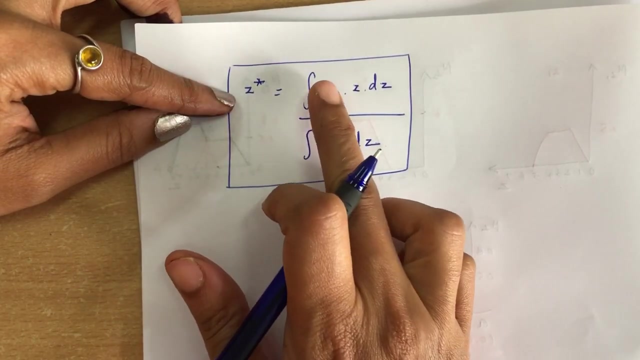 integral value. Integral value will be between 6 and it is ending at here. integral value is 6 here and ending at 8. So I am writing here: integral value will be 6 to 8.. Okay, So centroid formulas, z star will be algebraic integration of membership value of z into 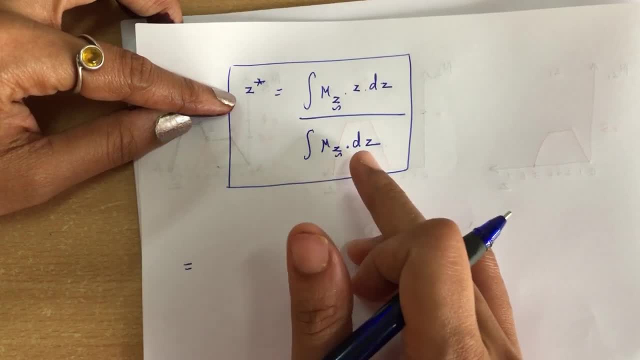 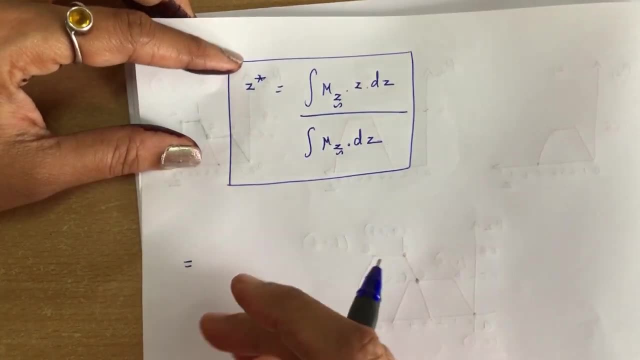 dz divided by algebraic integration of membership value of dz. So we will substitute all the values and we will find out the centroid value. So it is nothing. but so, since we have found out, we have already found out the straight line. 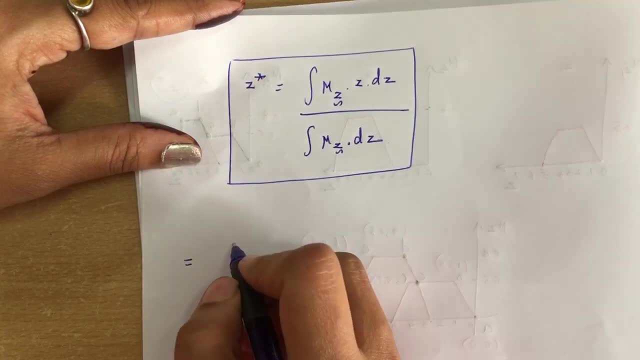 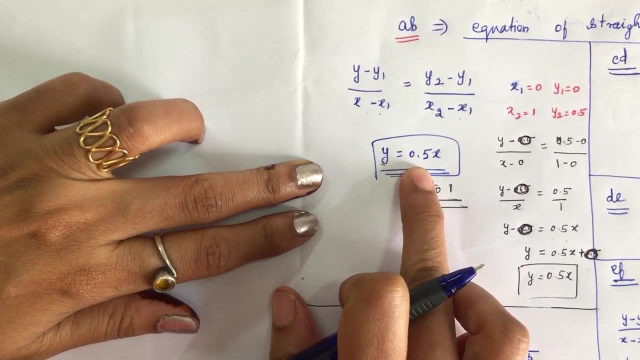 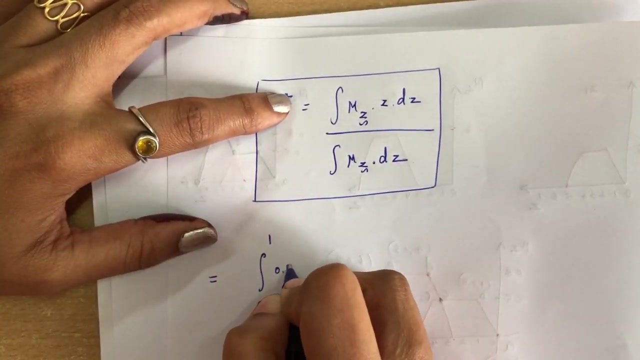 Equation for all the points. we will try to substitute all this thing. So the first equation, it is: first, it will be 0 to 1.. It starts from 0 to 1 integral and it is having a value called 0.5x. So we will write over here as this membership value is 0.5.. Okay, x is nothing but. 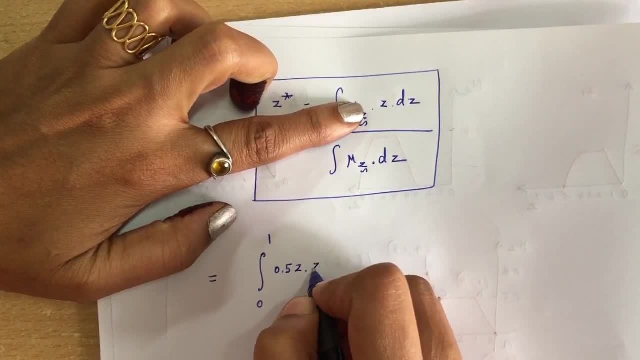 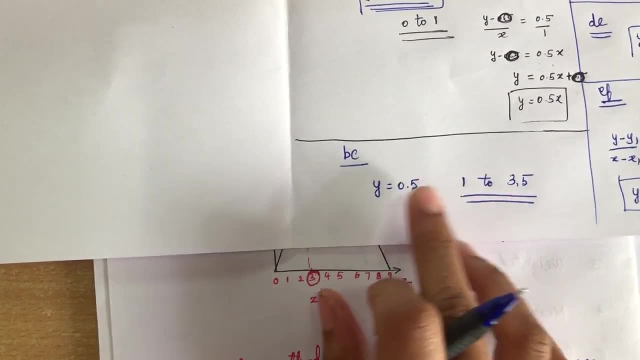 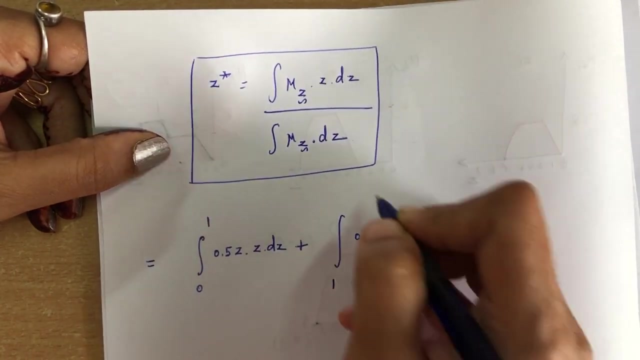 I am writing here z over here Already, z dz is there. I am substituting this thing. Okay, The second equation is from 1 to 3.. The value is y equal to 0.5.. So I will substitute here y equal to 0.5 and the value is 1 to. 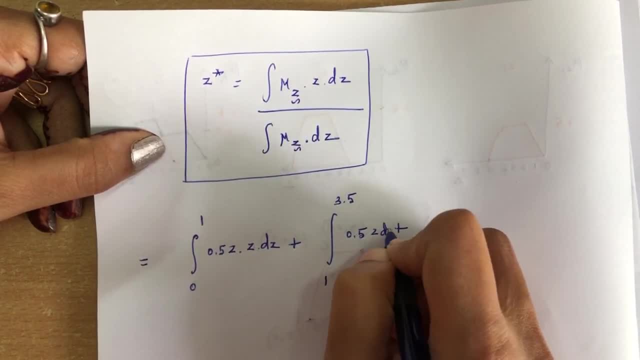 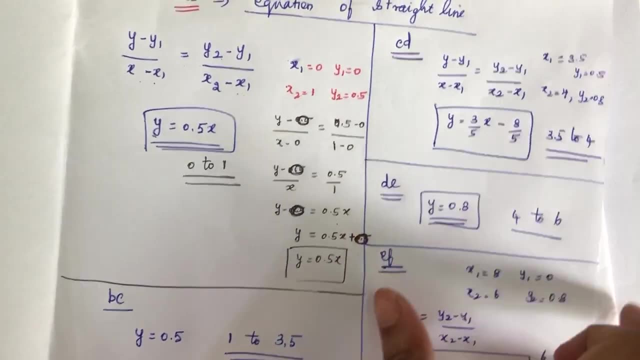 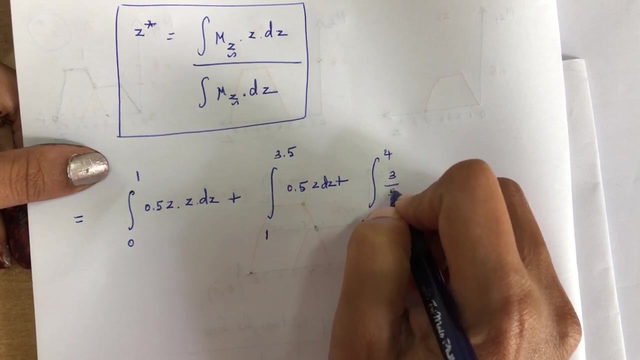 3.5.. Okay, Into z dz. and third equation is this one: 3 by 5x minus 8 by 5.. The integral value is 3.5 to 4.. So I am writing here 3.5 to 4.. So the formula is 3 by 5 into z minus. 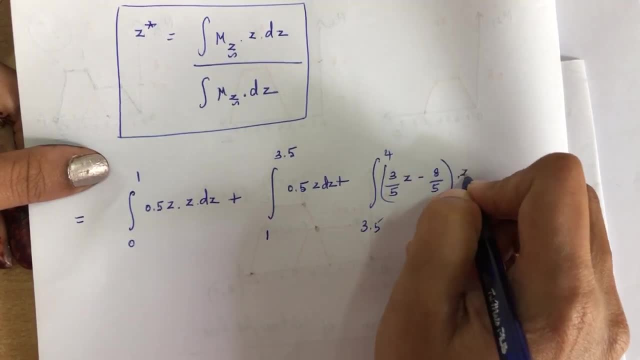 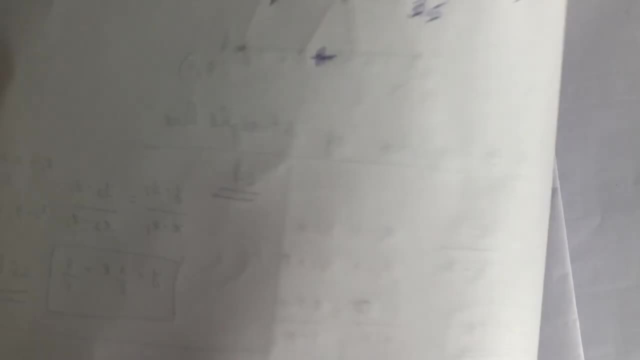 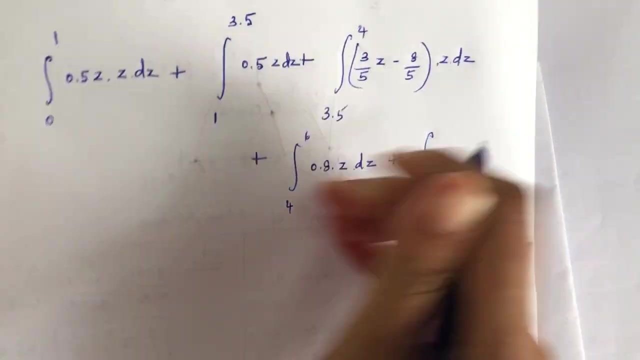 8 by 5.. Okay, Into z, into dz, Okay Plus. next equation is y equal to 0.8, 4 to 6.. So it is 4 to 6.8 into z, into dz. The last integral is from 6 to 8 minus 0.4x plus 3.2.. So I will substitute: 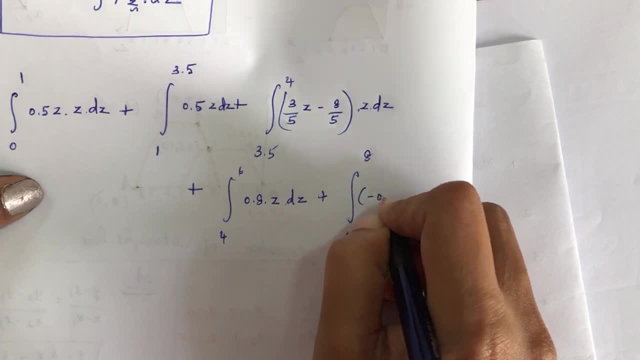 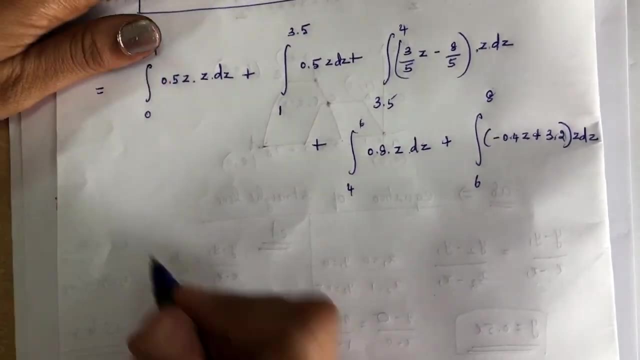 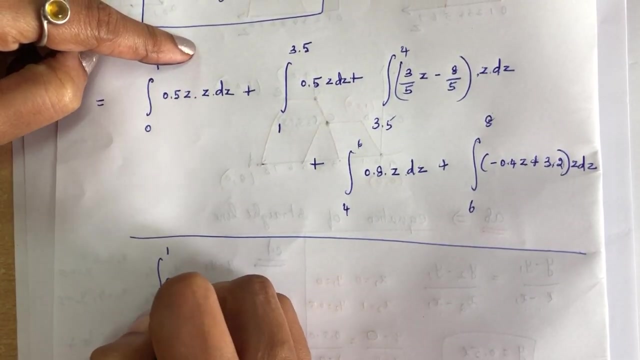 here it is 6 to 8 minus 0.4z plus 3.2 into z dz. Okay, This is what I am getting: the numerator, So the denominator value, the same thing I should write without writing this z. So it will be 0 to 1, 0.5, 0.5 into z dz plus 1 to. 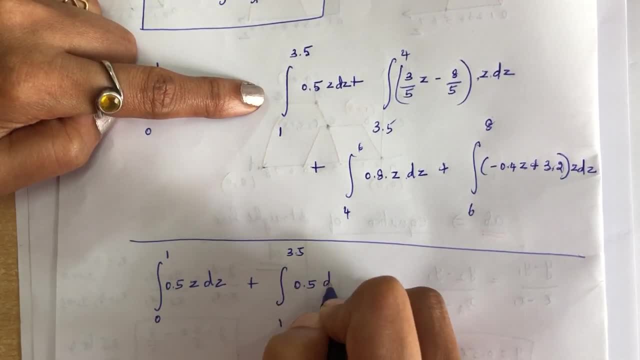 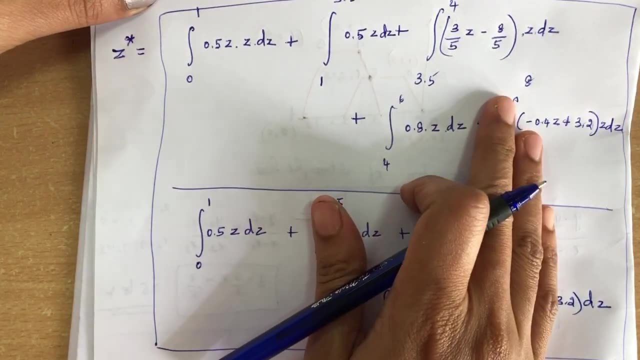 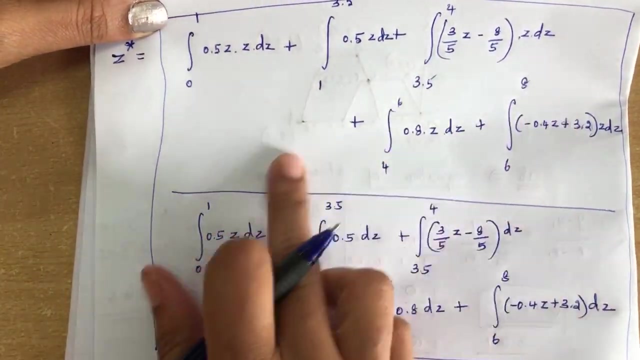 3.5, 0.5 into dz plus same thing. I will write it for everything. So this is what the final. when you substitute all the values over here, this is what the formula you will get. So now, when you solve all these numerator and denominator, you will get the value as 4.151. 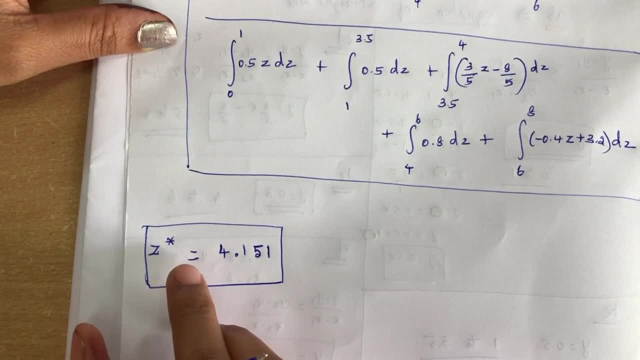 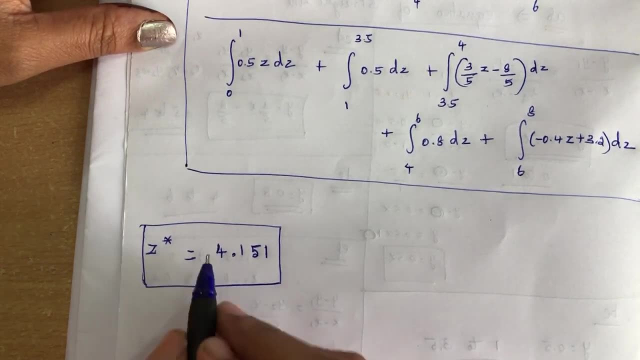 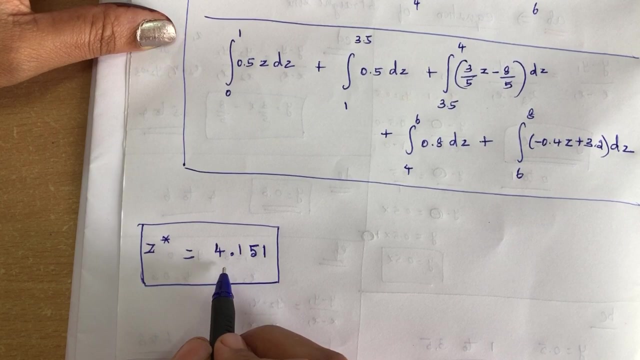 This is how you will convert your fussy value into de-fussified value. This is your de-fussified value. So you have used centroid method for converting your fussy value into de-fussified value, So final output for this particular de-fussified value is 4.151.. Okay, So this will be in between 4.151 and a. Okay, So this will be in between 4.151 and a. So this will be 4.151 into D Fussy. Okay, Now you go back tommmunt. This is the word. 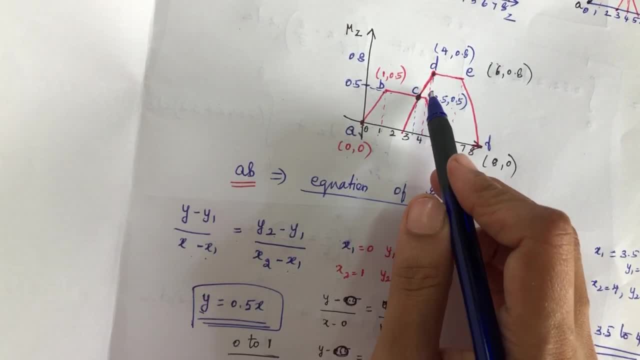 form for médiaimal. So you were writing this and this was降th. Now you could write K and D rootów 4.151 for your. the centroid value will be between 4.151. this is your output for the for finding for. 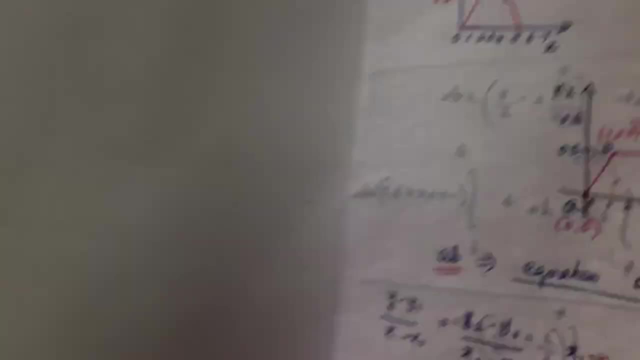 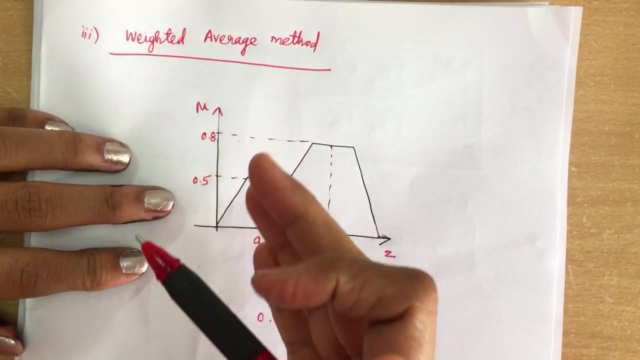 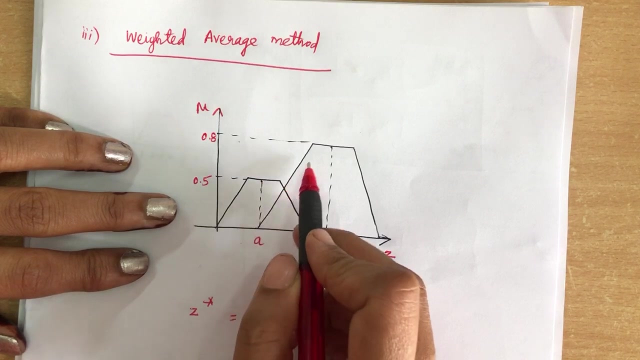 converting your fussy value into defussified value. okay, Moving on to the third method, weighted average method. in this weighted average method I will explain with an example. then I will go explain the equation for this weighted average method. so in this diagram I have taken two fussy 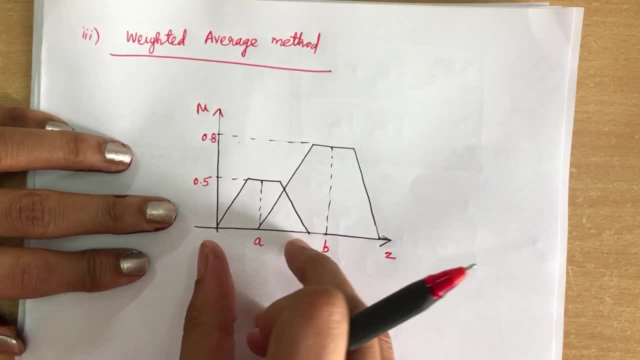 sets. I have taken the union of two fussy sets, let me call it as this particular fussy set is having a center value called a and for this particular fussy set I am having a center value called b. okay, So the membership value, the maximum membership value for this particular fussy set, is: 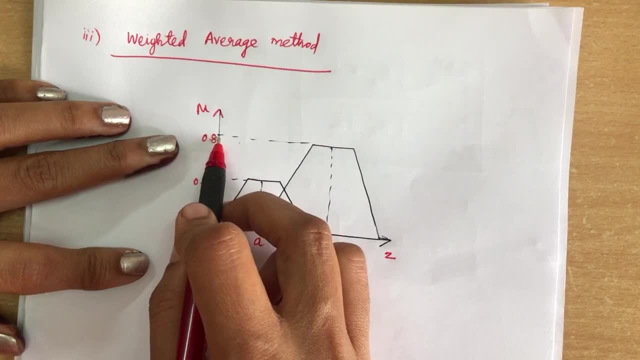 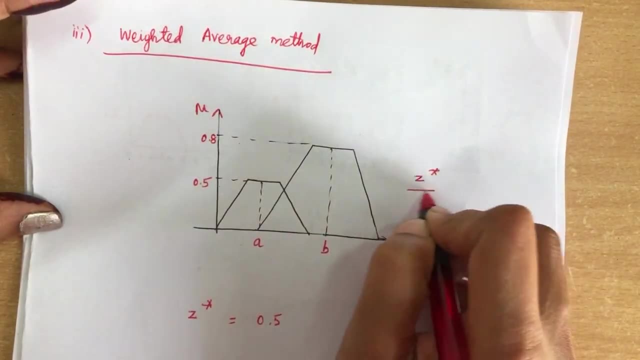 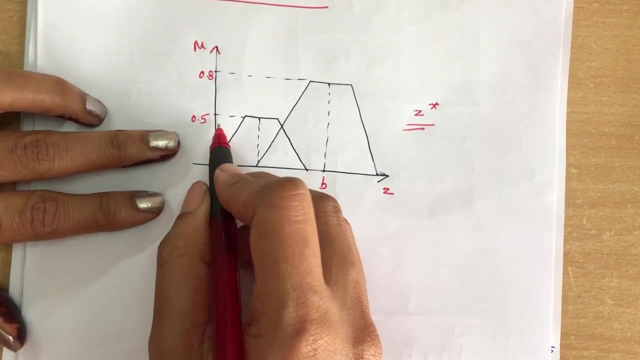 0.5 and this particular fussy set is 0.8.. So, by using weighted average method, I need to find out the defussified value called is it star. So how do you do this particular weighted average method, That is, z star is given by 0.5- this is the membership value, 0.5- into the center of this. 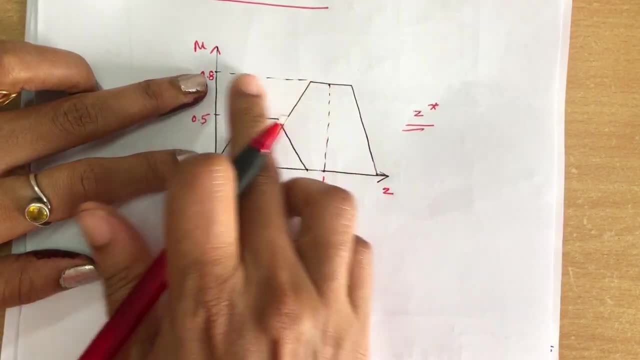 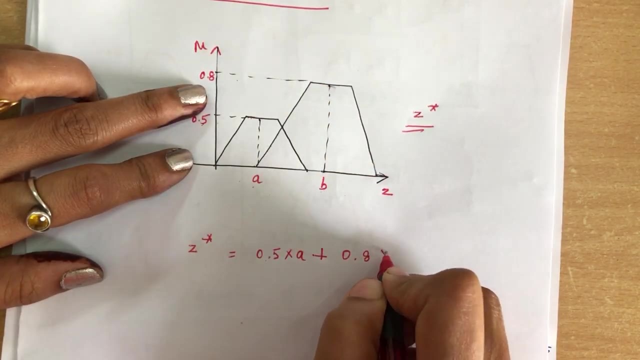 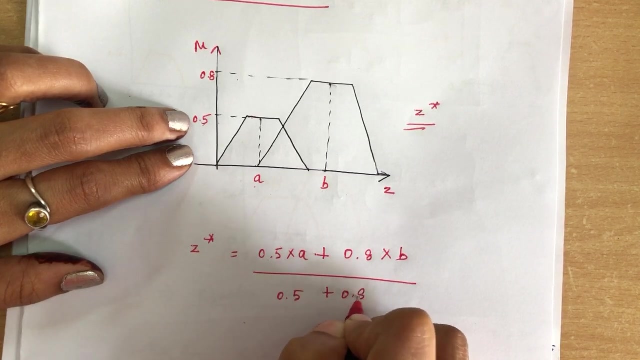 particular value. okay, plus, and what is the membership value for this particular fussy set? it is highest membership values: 0.8. 0.8 into the center values into b. divided by this membership values, that is nothing but 0.5 plus 0.8. okay, this is the formula for finding out the defussified. 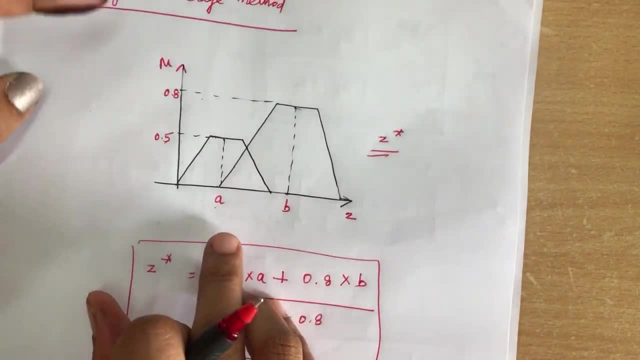 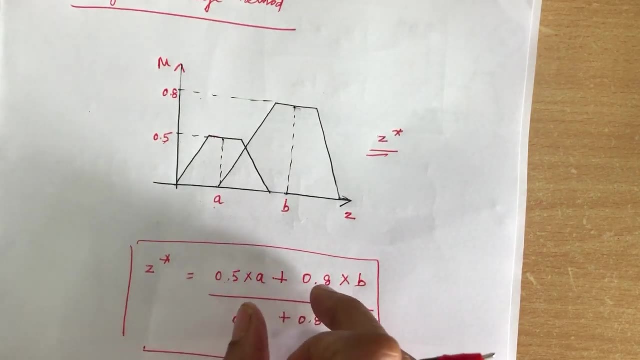 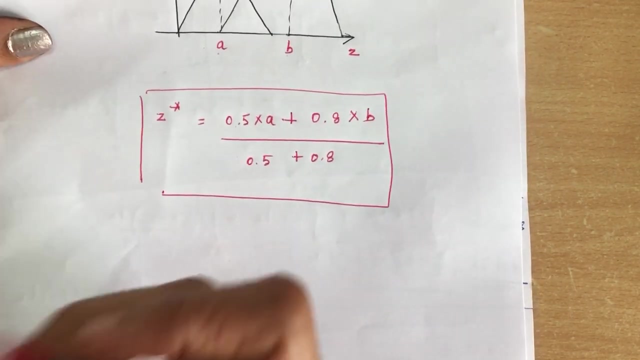 value using weighted average method. So you have to multiply the membership values into the center of the value. it is like algebraic sum of all the membership values into center of the values divided by the summation of all the membership values. okay, We can write in general. we can write. 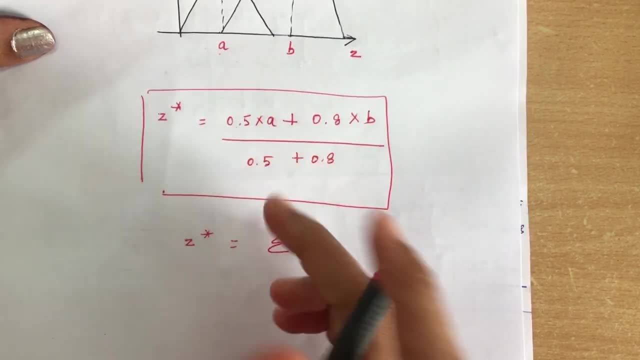 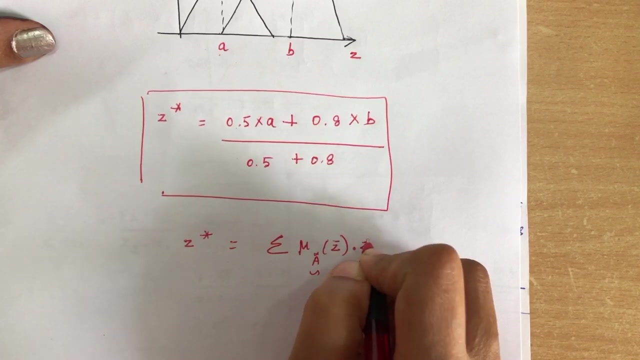 this as an equation, that is an algebraic sum. this is here algebraic sum, so I am using the summation method. okay, membership values of this particular set. I am giving the naming it to be a bar. okay, a delusible. okay, a into z bar. into z divided by algebraic summation of z bar. 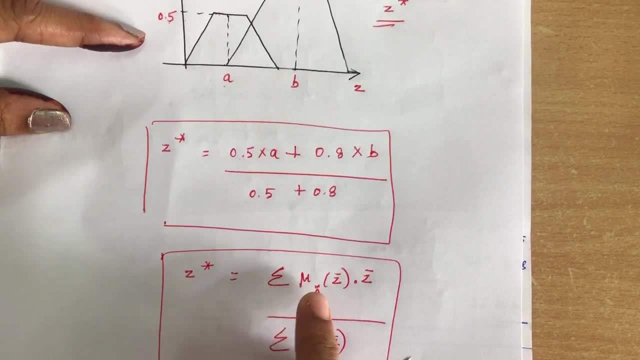 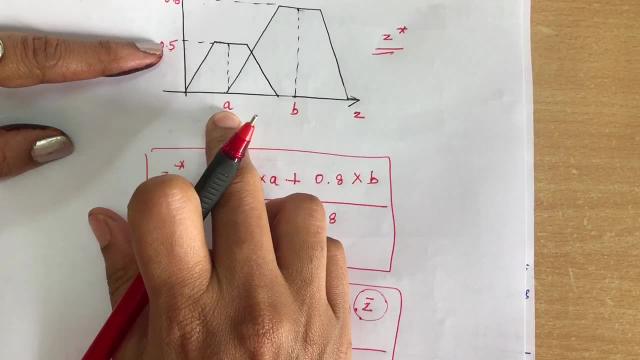 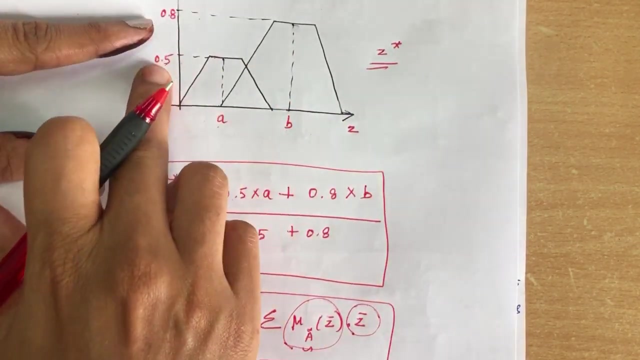 okay, so this is nothing but the membership values. this is what your membership value and this is your center value. okay, that is what membership value into the center value of first fussy set, plus membership value into the center value of your second fussy set. that divided by all the membership values. 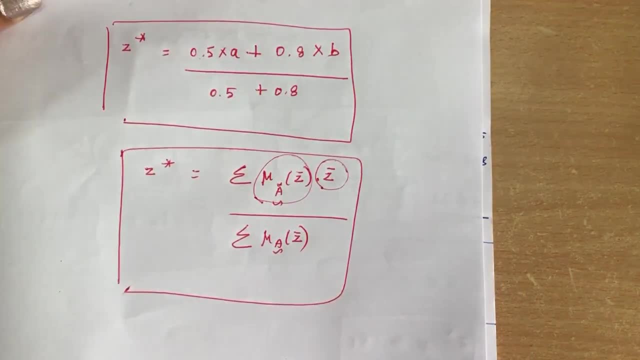 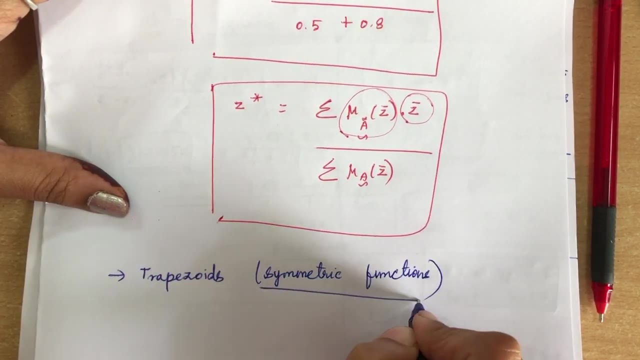 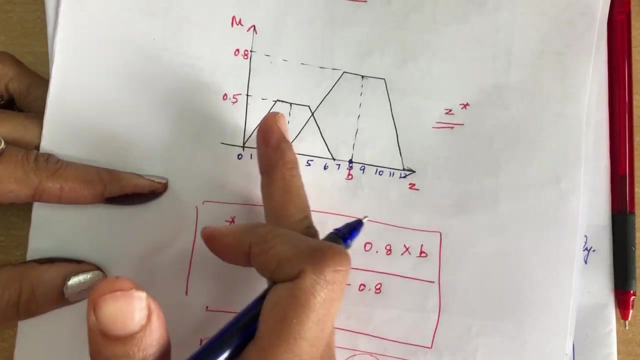 That is what I have written, the general equation, okay. So one thing you have to note in this weighted average method is: this particular method will be applicable only for symmetric functions. so here I have taken a trapezoidal function which is symmetric in both the sides. so this particular 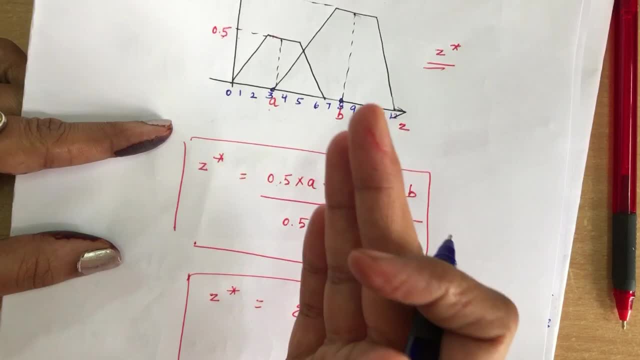 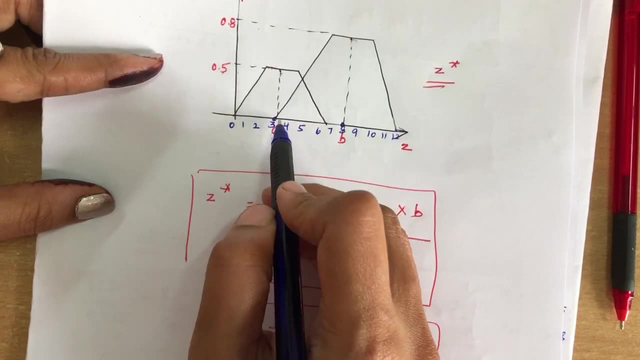 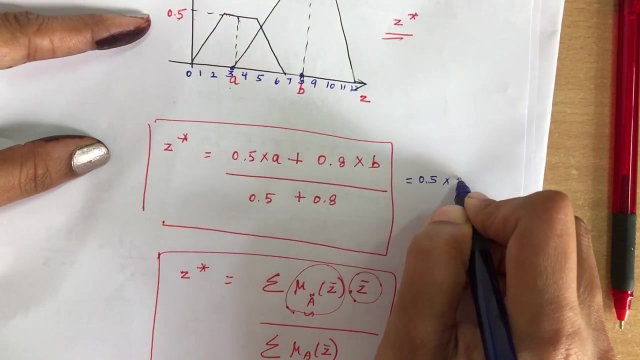 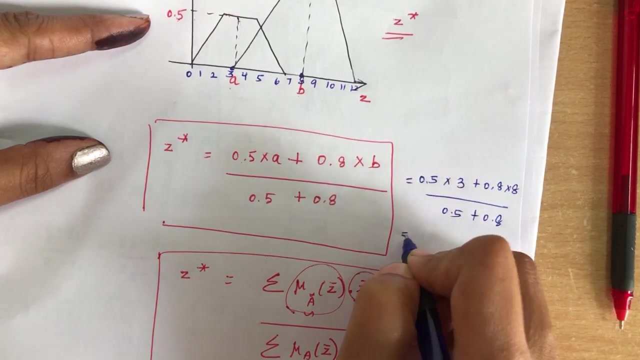 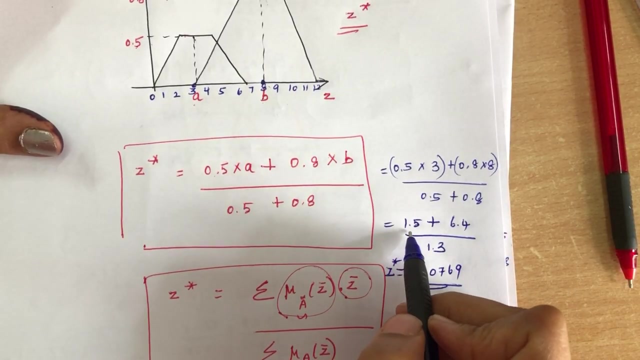 method will be applicable only for symmetric functions, then only you can use this particular method. So, for example, we will find out the answer for this. so here the a point I am giving here 3, and b point is 8. so when I substitute here, I will get 0.5 into 3 plus 0.8 into 8. завutenNote. 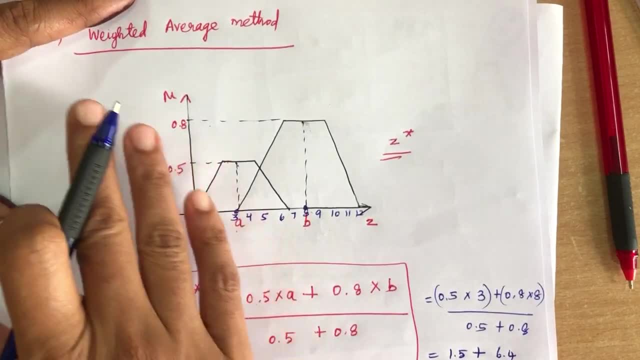 2. 5 지금까지. b point is 8. so when you substitute here and get .5 into 3 plus .8 into 8, du per five plus .8, okay. So I will substitute from the values and get the. 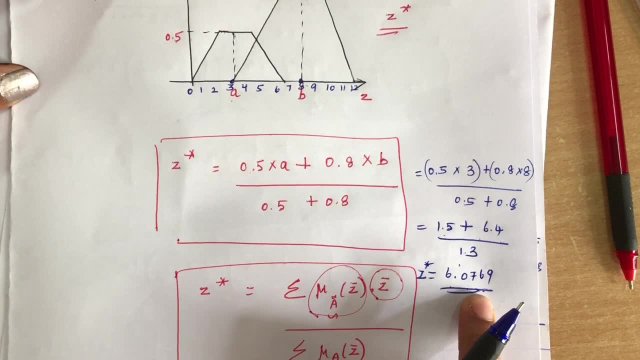 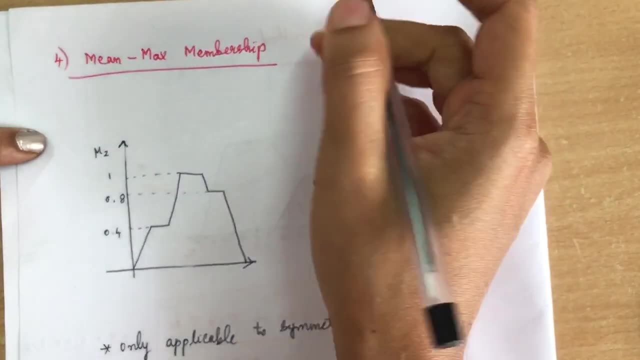 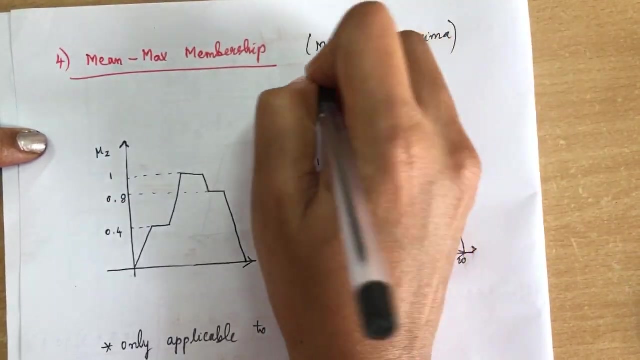 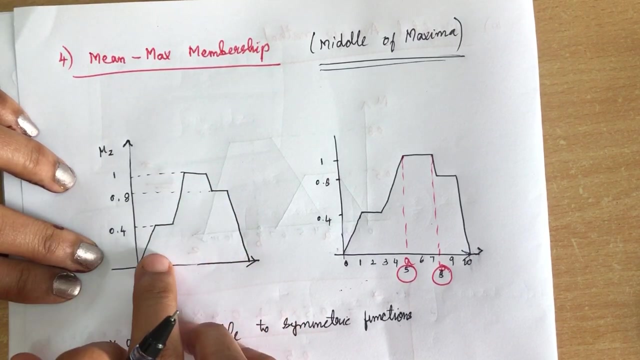 formula i am getting to be 6.0769. okay, moving on to the next method, mean max membership principle. it is otherwise called as middle of maxima, so by the name itself you can understand that we are going to find out the middle of the maximum membership function. so here i have drawn a fussy set which is formed by: 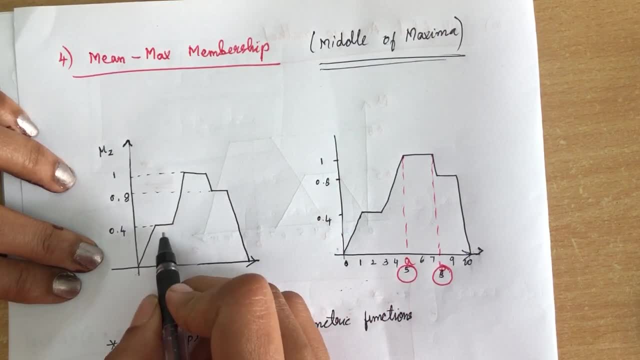 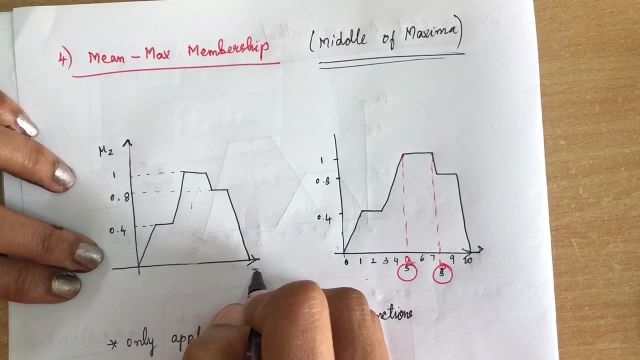 combining the union of three fussy sets. okay, so you combine three fussy sets. i am getting this particular fussy set now and i am here. i am going to have this particular fussy set- x axis, i am calling this. is it in y axis? i am taking the membership value and it is having a peak value. 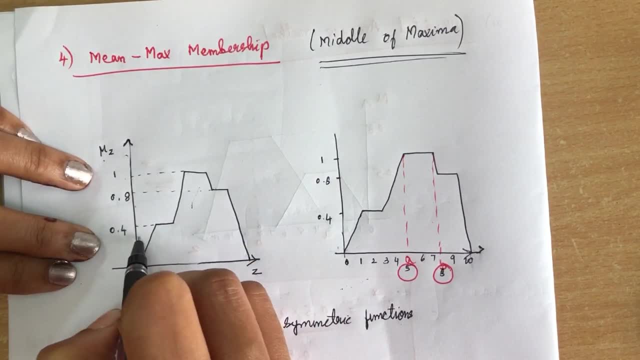 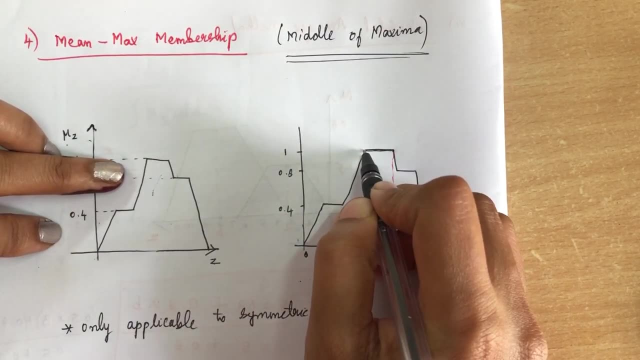 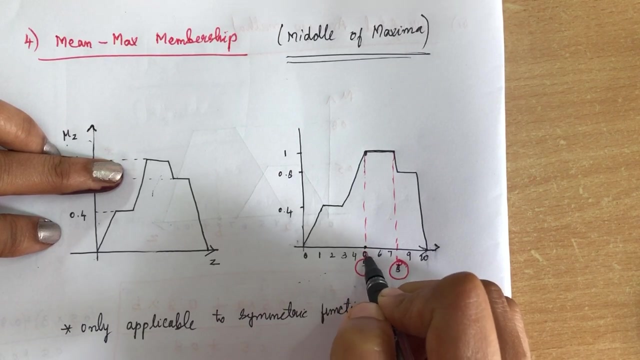 at 1, and then 0.5, 0.8, and then over here 0.4. okay, so what is mean max membership function? so here the among the membership value, you have to take the mean value. so this side it starts. i am going to extend this particular point and here i am getting this. 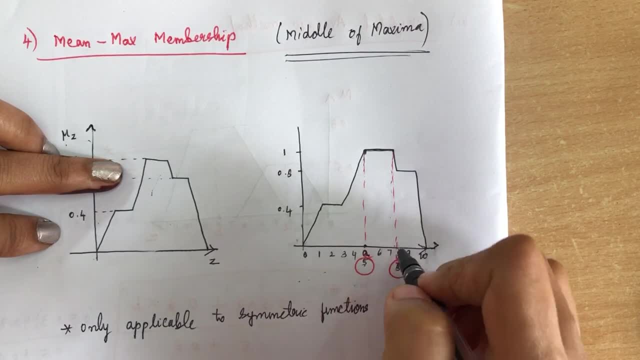 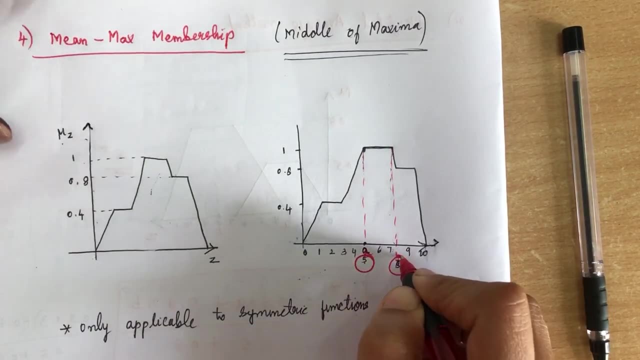 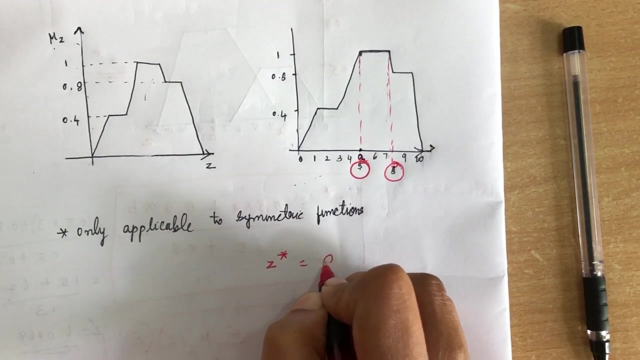 particular point as a and this particular point i am extending over here down. i am getting this point to be b. okay, so this value is a and b. so the formula for this mean max method, that is, is it star? is it star, will be a plus b by 2. that is, when i solve this example, i will get 5 plus 8 by 2. 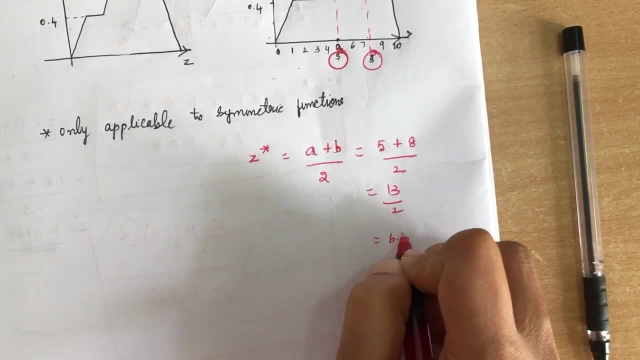 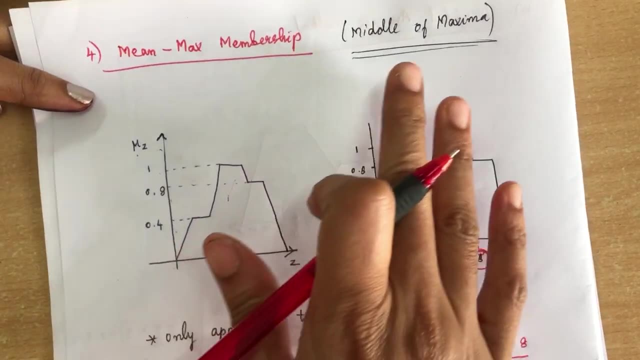 that is 13 by 2, that is nothing but 6.5. so that is this is your d for c5 value. so for mean max method, it is very simple. it is nothing but middle of maxima. so i need to find out the, the middle value in your. 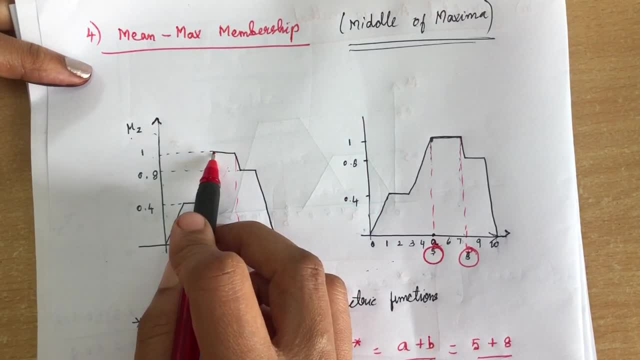 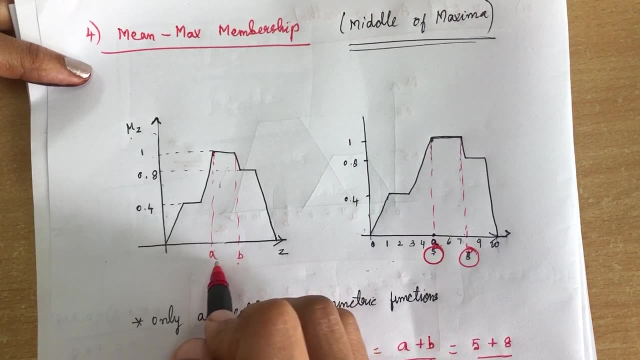 maximum membership function. so what is your starting membership value, the maximum membership value? it starts at point a and it's n set b, and i need to find out the middle value among the two membership values. so it is nothing but a plus b by 2.. 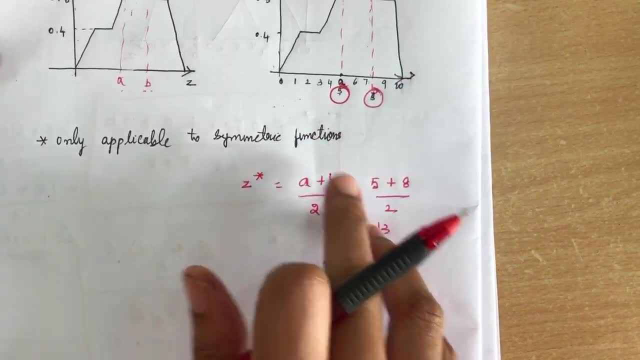 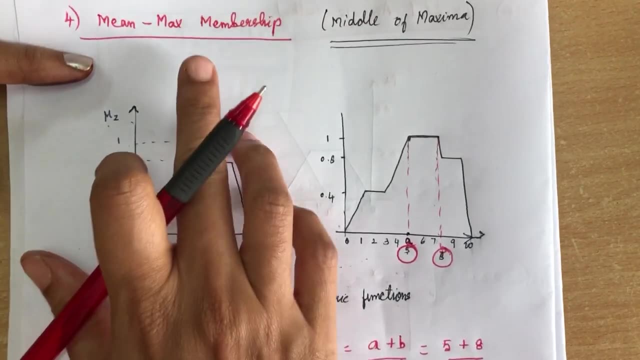 so this is the formula for finding out the mean max membership function. so when i substitute 5 plus 8 by 2, i am getting here 6.5. this is your d for c5 value. but one thing over here in mean max principle is it can be applied only for your symmetric function. so here i have taken only 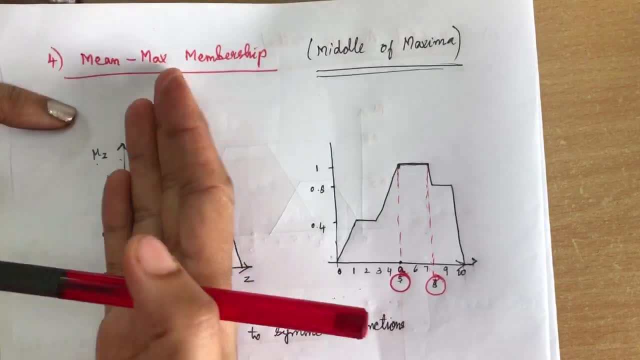 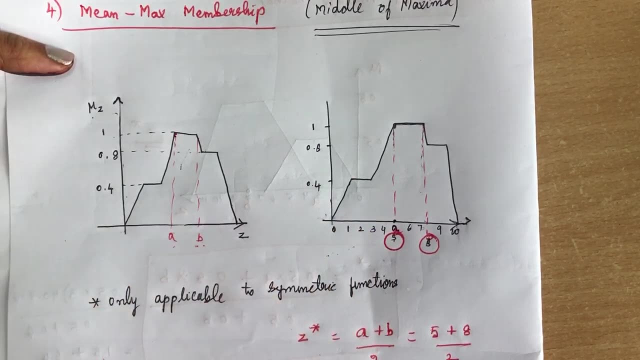 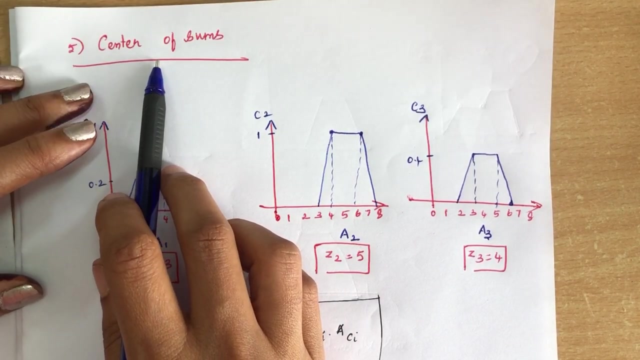 trapezoidal function, since it is symmetrical, so i can apply this particular method for these particular functions. so you need to find out which method you have to use for any particular. okay, moving on to the next method center of some method. so by using this method we are going to find out the d for c5 value. 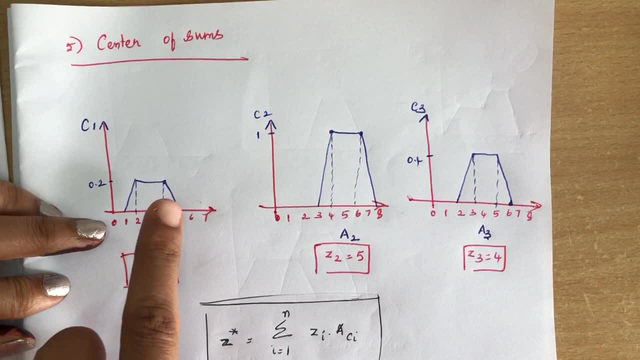 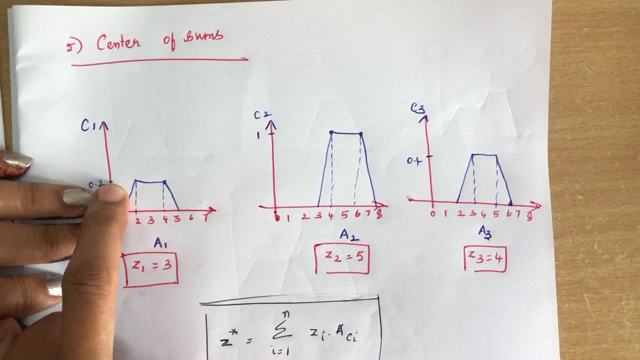 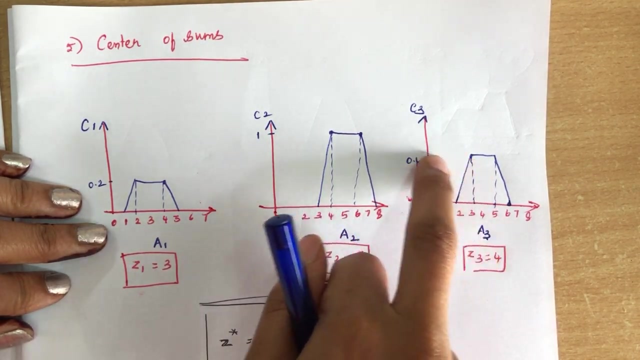 so here you can see the three diagrams i have drawn. so the first diagram represents c1 and c2, and this is the c3 and c1 is having a maximum membership value called 0.2 and c2 is having a maximum membership value 1 and c3 is having a maximum membership value 0.4. you can see in this: 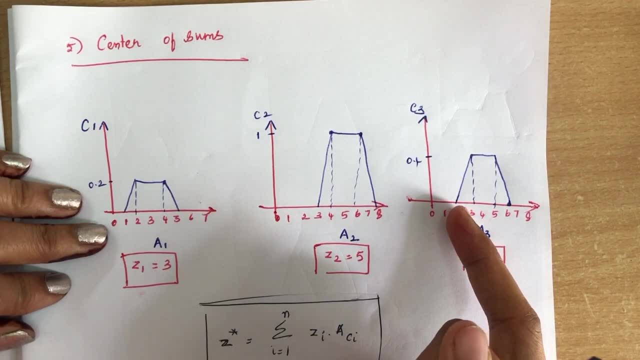 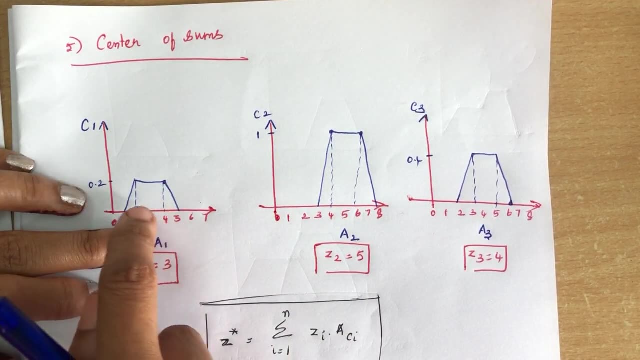 diagram. all the diagrams are trapezoidal functions i have used. so in this center of some method, i need to find out two values. one will be the area which is bound by this particular region, and then i have to find out the center, geometrical centers. 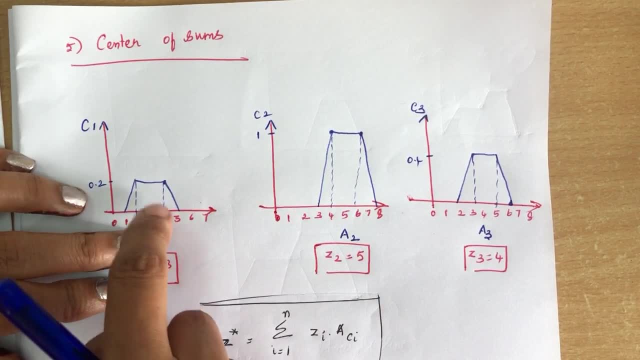 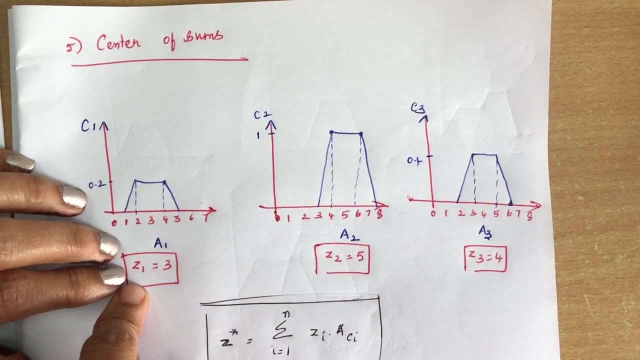 of this particular region. so this a1- i represent the area of this particular, this particular set- and a2 and this, i'm naming it as a3 and what is a geometrical center for this particular set? so the geometrical center it is having at 3, okay, is it? 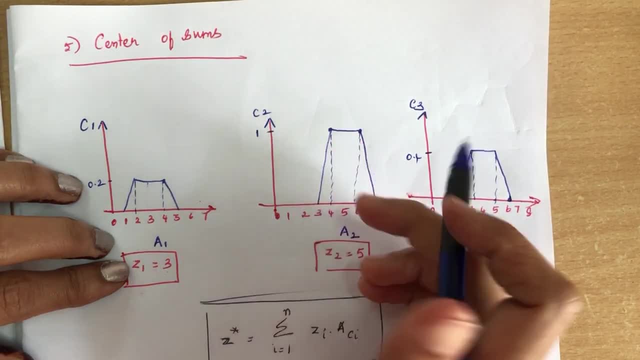 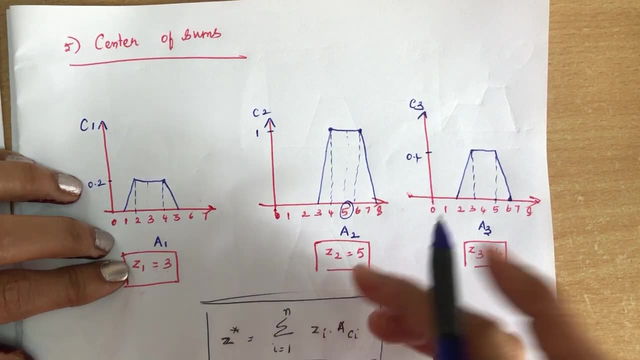 1. i'm naming it to be. is it 1? is it 1 is 3, and for this particular region, the geometrical center is 5. so naming to be: is it 2? it will be 5, and for this it is 4. okay, is it? 3 is 4. so the formula for 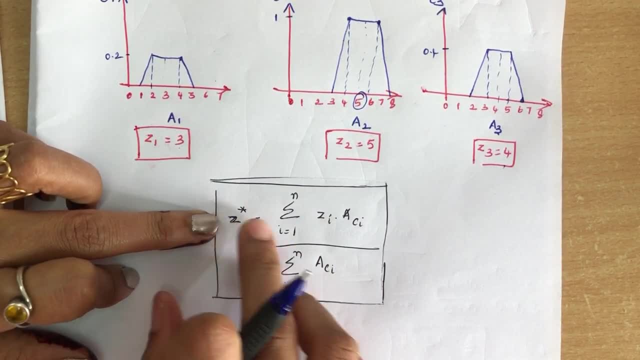 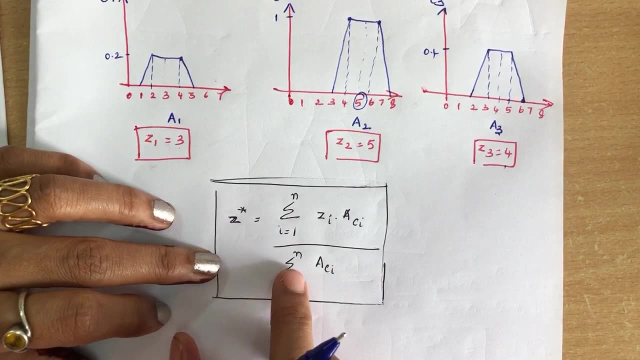 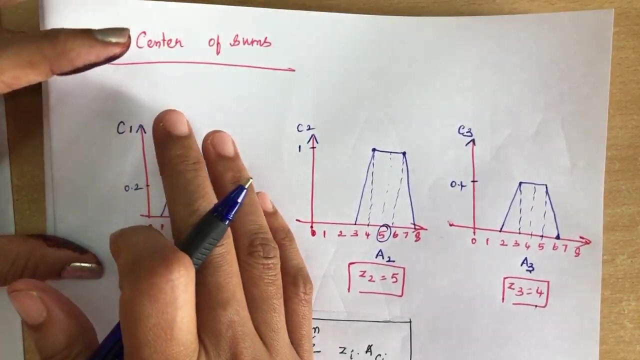 the center of some method will be d. specific value. is it star will be algebraic summation of i equal to 1 to n. is it i into the area divided by algebraic sum of i equal to 1 to 1 divided by the area. so this is the formula for finding out the center of some method. so we will substitute: 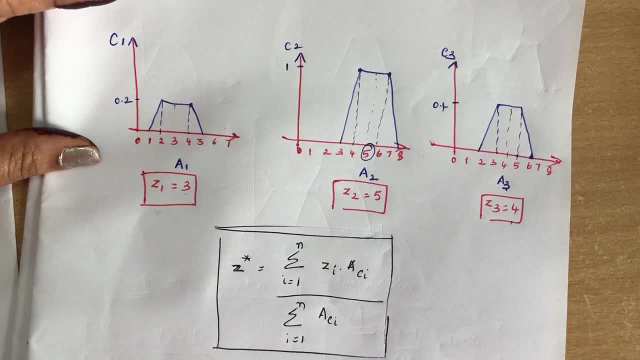 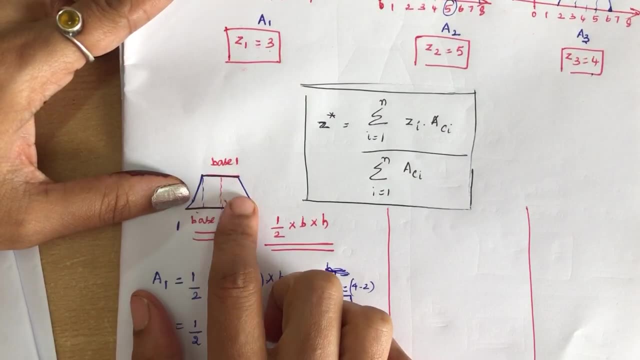 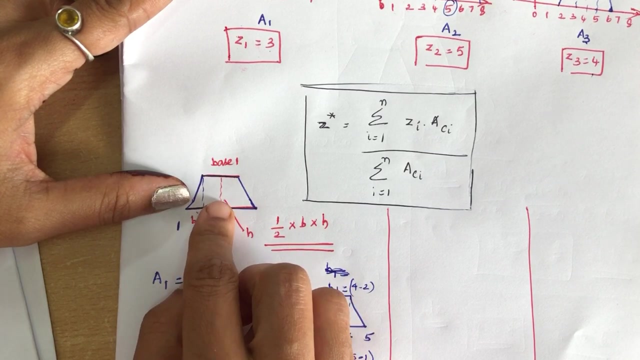 all these values and we will find out the d specified value. okay, so first i need to find out the area of this particular fuzzy set, c1. okay. so what is the trapezoidal? how do you find out the trapezoidal area? so area will be of into b, into h. h is the height over here and b is you are having. 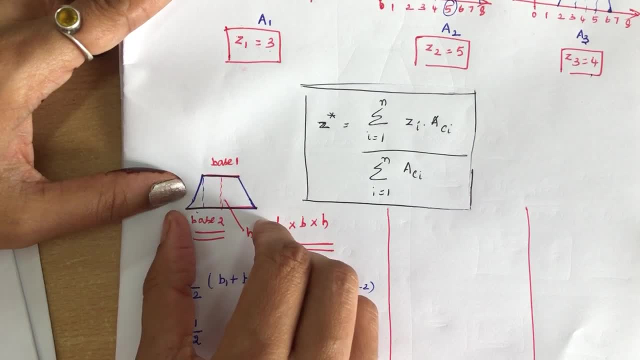 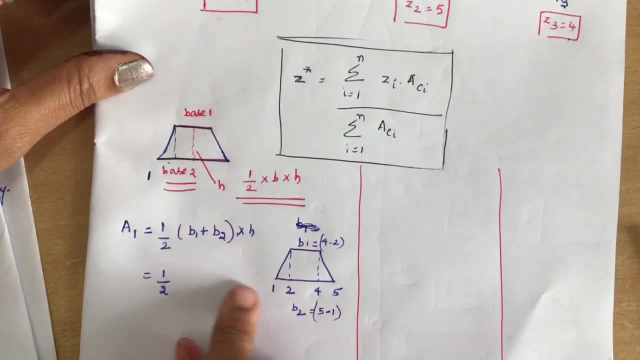 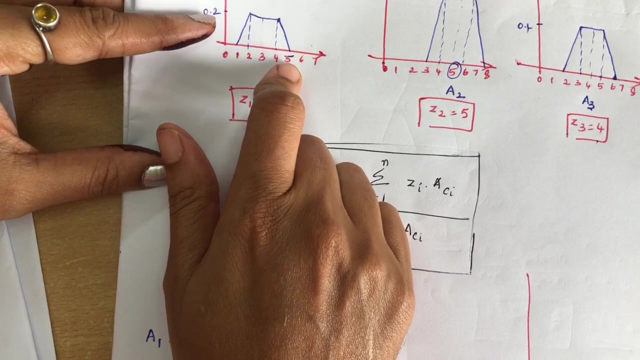 two base over here. the base one is the smaller one and base two is the larger base. okay, so first we will find out the fussy set, the area for this particular region. so for this particular region i have drawn here same thing: 1, it starts from 1 and 2, then 3 and then it's n set. 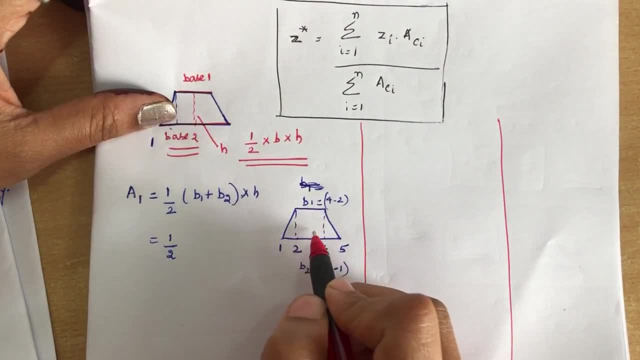 5. okay, the same thing i've drawn over here. so base one is 4, base one. how do you calculate this base one? it is nothing, but it's n set 4 and it starts from 2. that is nothing, but 4 minus 2. that will be. 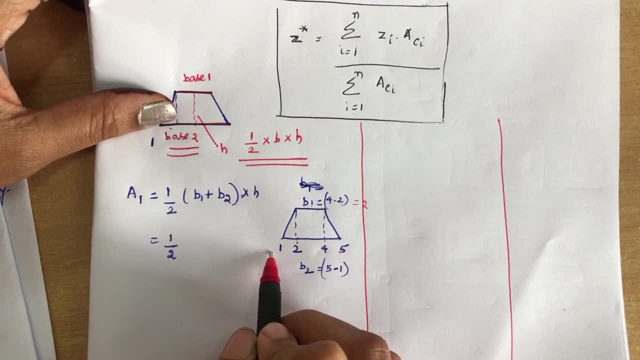 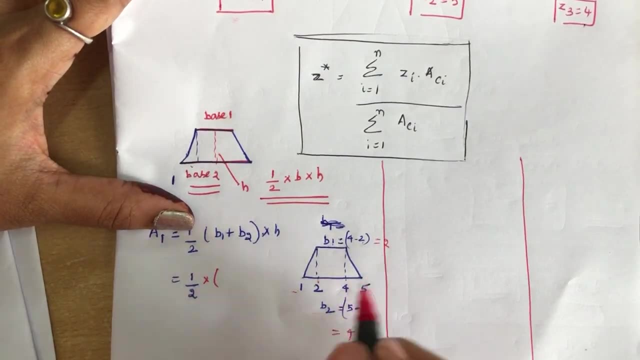 2 and for the base 2 it is ending at 5 and the distance between 1 and 2 is the distance between 1 minus 5, that is, 5 minus 1, that will be 4. so i'll substitute here 1 by 2 into b1 is, 2 into b2 is. 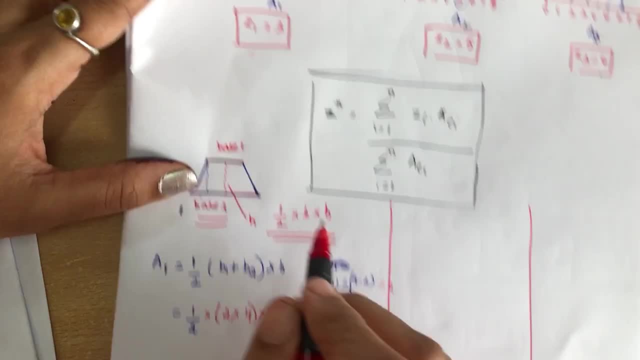 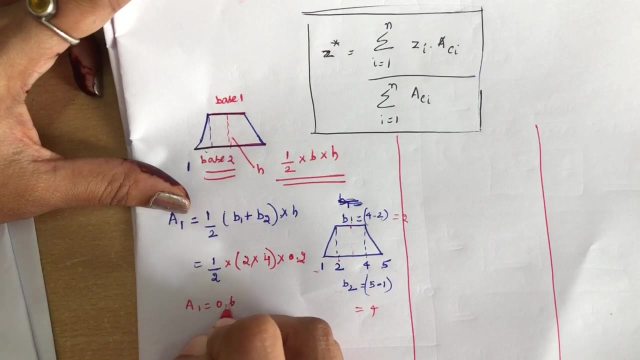 4 into height is. height over here is the same thing. height over here is 0.2 into 0.2. so when i substitute here a1 i'm getting to be 0.6. the area of for this particular region is 0.6 the. 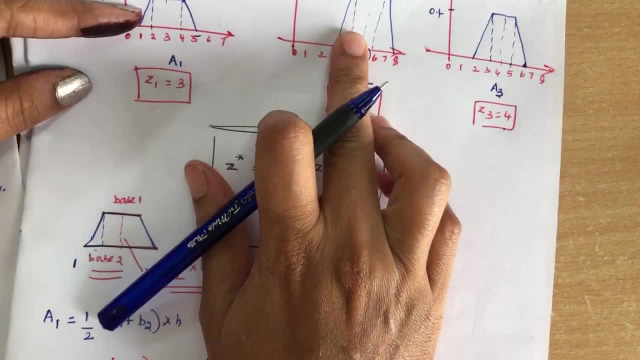 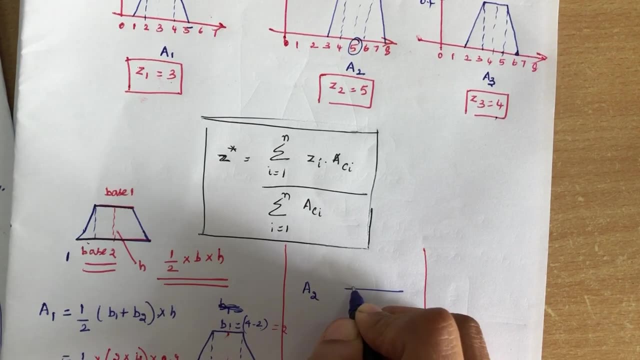 same thing. i'll find out the area for this particular trapezoidal also. so how do you find out the trapezoidal for this a2? a2 will be so it is okay. so it starts from 3 and here it is 4 and here it is 5, 6 and n set, 8: n set. 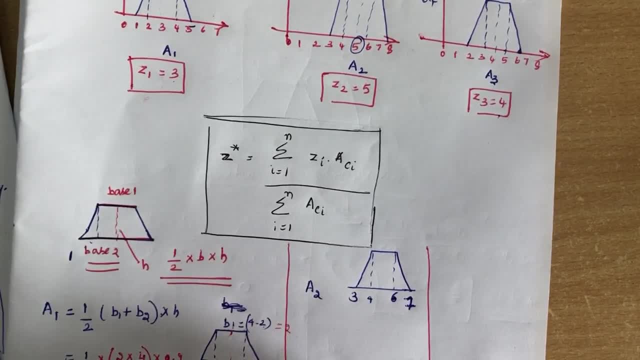 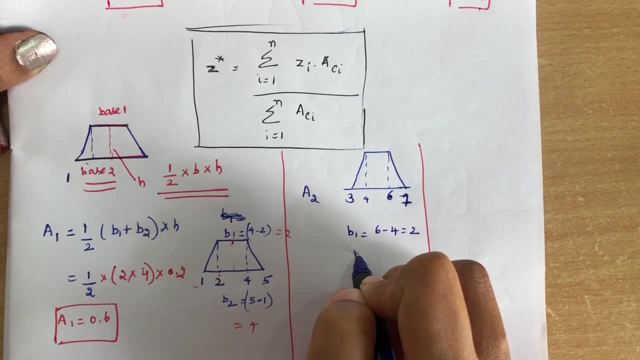 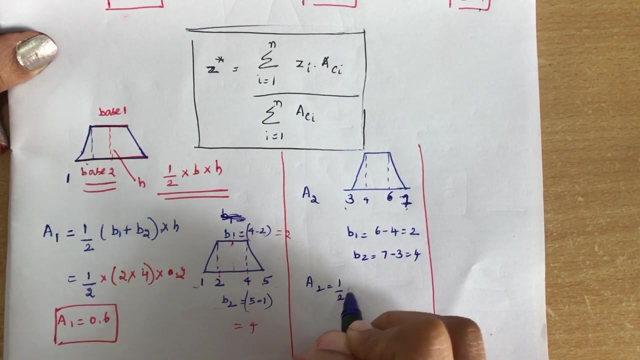 7 n set 7. okay, so what is base 1? this base 1 will be 6 minus 4, that is 2. base 2 will be 7 minus 3, 7 minus 3, that is 4. so substitute here lif, Which is 2, i have x2, so we find out the. 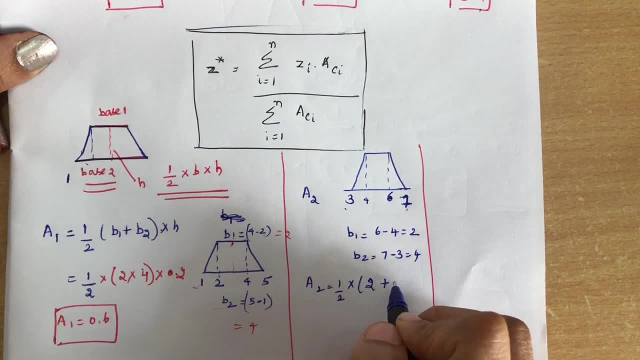 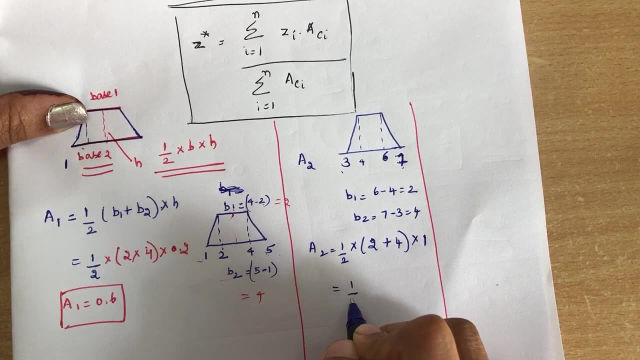 the time 1 minus 4, it is 3av. So if times is x2?, 2 is equal to the time we have in here, x2. And how come? so你的1b2å rescue A2 will be off into b1 is 2, plus 4 into what? 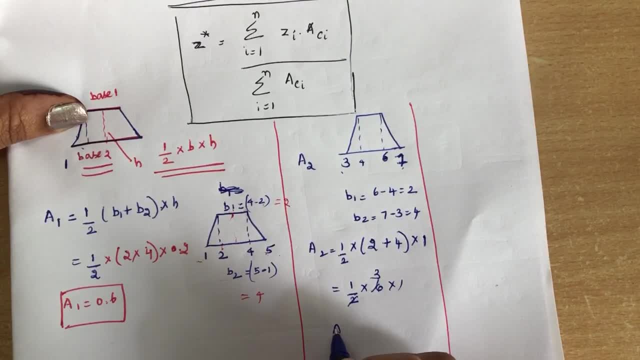 A1 will be off into b1 is 2, plus 4. into what sis this membership value? What is this membership value? That is 1. okay, That is 1. so you will get 1 x 2 in to 6 x 1,. 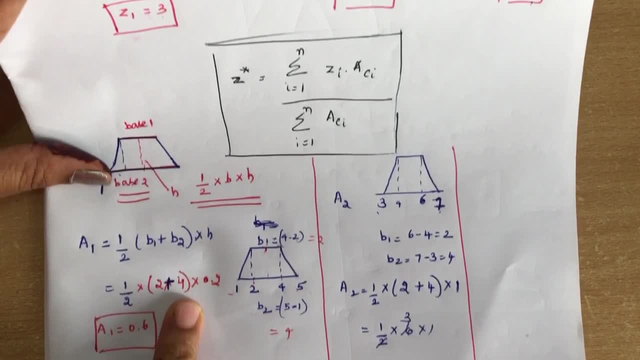 that is nothing but 3, A2 will be equal to 3.. Okay, here it is plus 7.. 2 plus 4 into 2 plus 4. i have written here multiplication, here b1 plus b2, that is with: 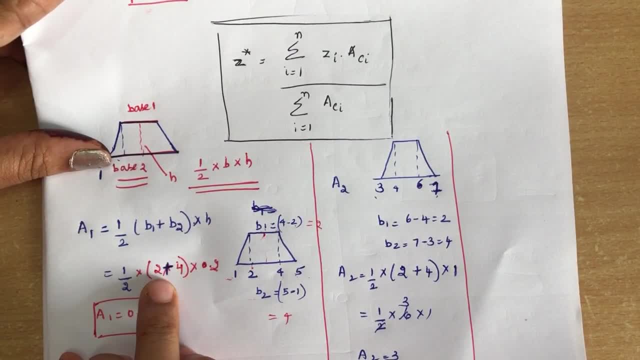 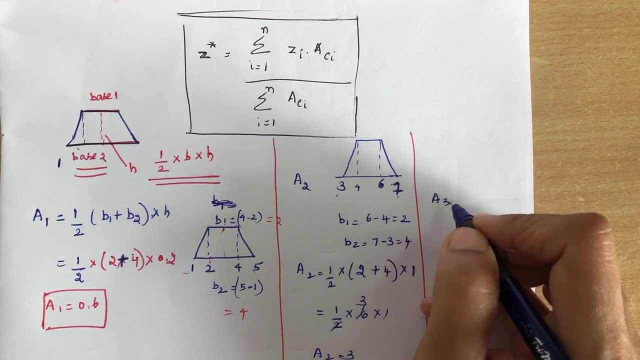 here you have to, and here b1 plus b2, that is 2 plus 4. i have to write it. you have to. here: b1 plus b2, that is 2 plus 4, okay, So now we will draw it for a3. So. 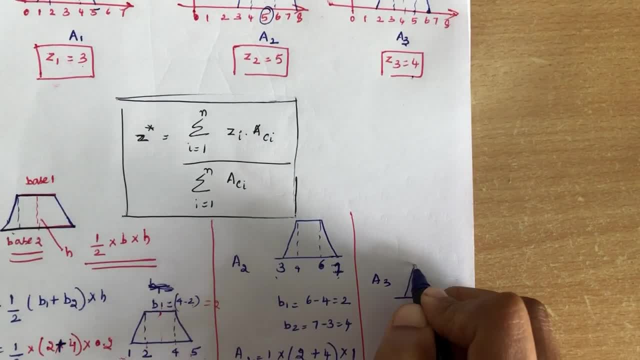 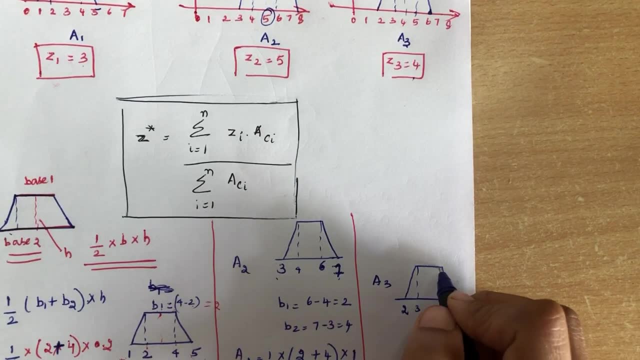 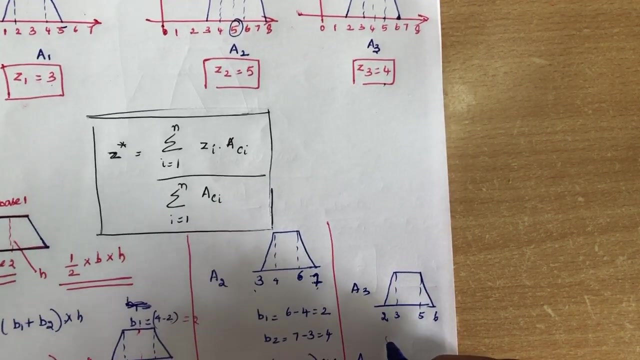 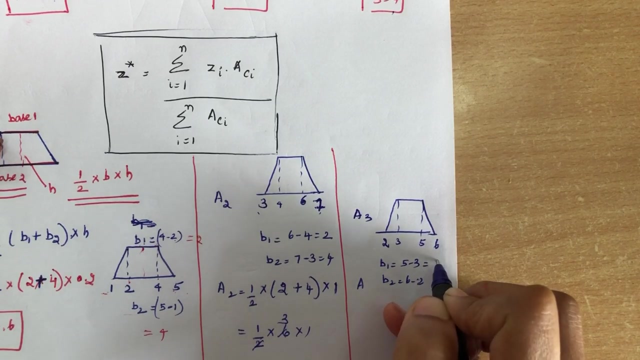 what is a3? Start from 2 and then 3. here and here it is 5 and a ends in 6, okay, So that will be. so. what is base 1? here b1 will be 5 minus 3, b2 is 6 minus 2.. That will be here. 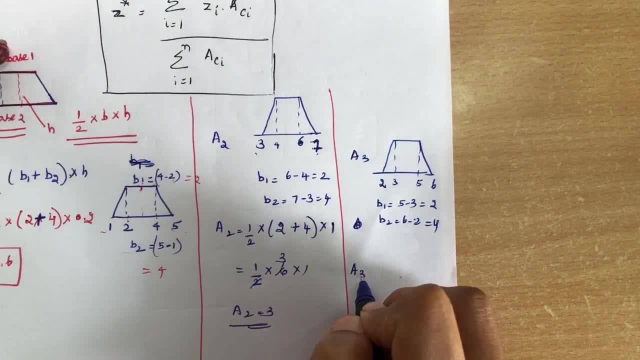 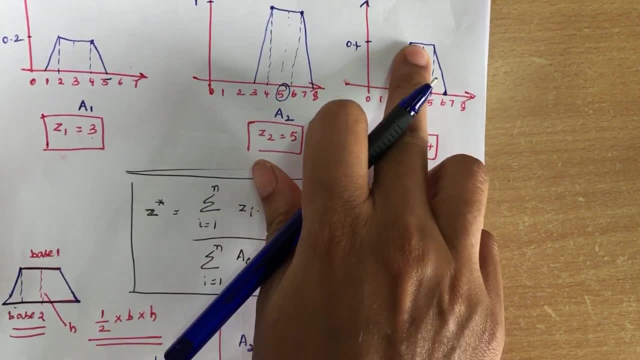 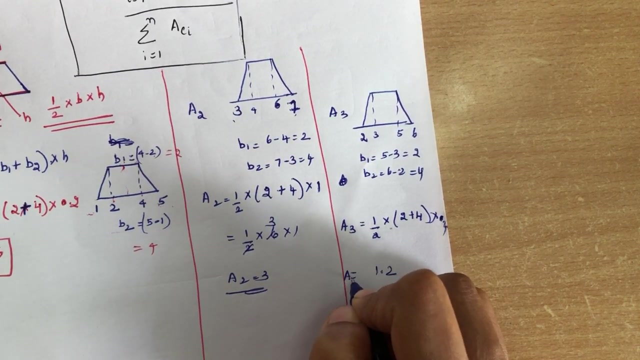 it is 2, here it is 4.. So a3 will be 1 by 2 into 2 plus 4 into what is the membership value height? It is 0.4.. Into 0.4, the answer will be 1.2.. So when I substitute this the 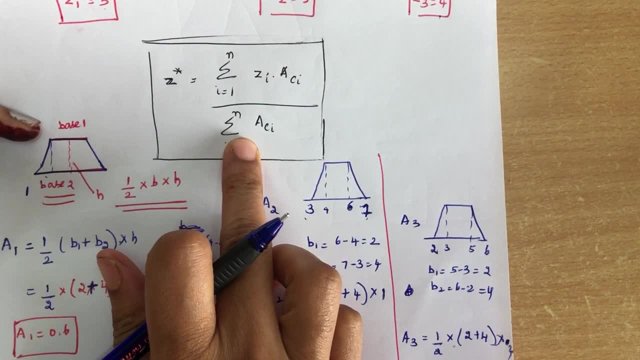 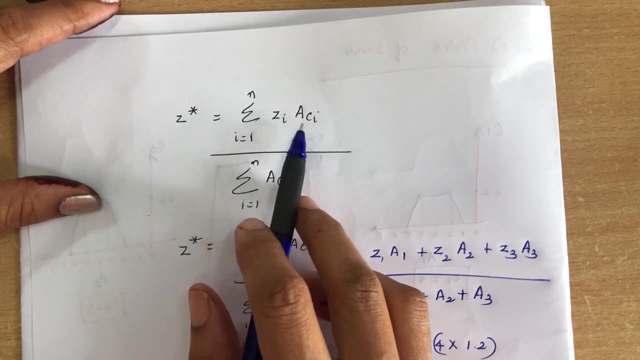 answer is 1.2.. So now we will substitute. We will substitute all the values in this equation and we will find out the de-facified value. okay, So the formula de-facified value will be sigma i, equal to 1 to n, zi into aci. 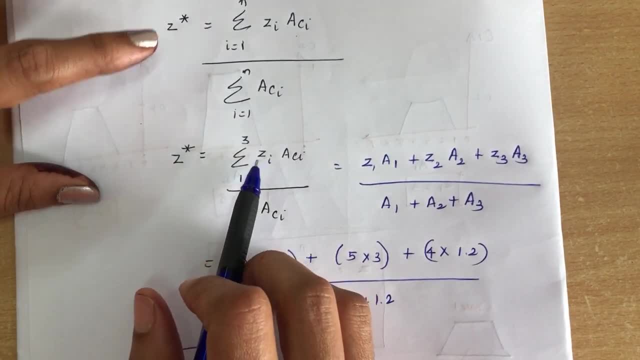 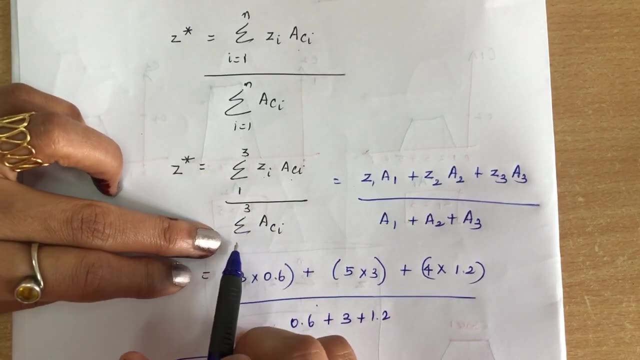 divided by sigma i is equal to 1 to an aci. So since there are 3 regions, so n will be 3 over here, sigma i is equal to 1 to 3, zi into aci divided by sigma i is equal to 1. 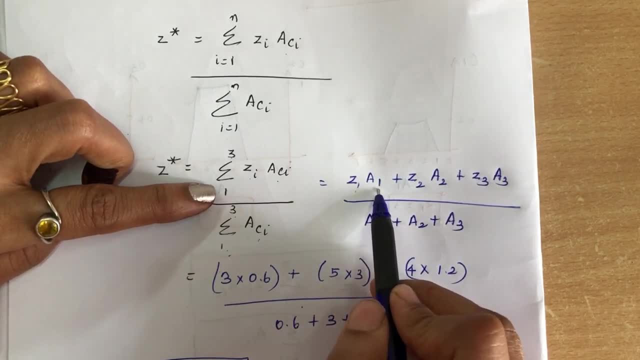 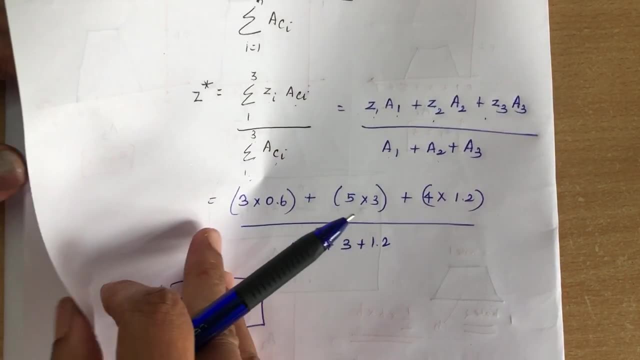 to 3 aci. So that is nothing but z1 into a1 plus z2, into a2 plus z3, into a3 divided by a1 plus a2 plus a3.. So what is z1? in the first formula z1 is 3 and z2 is 5 and z3 is 4.. So I will substitute: 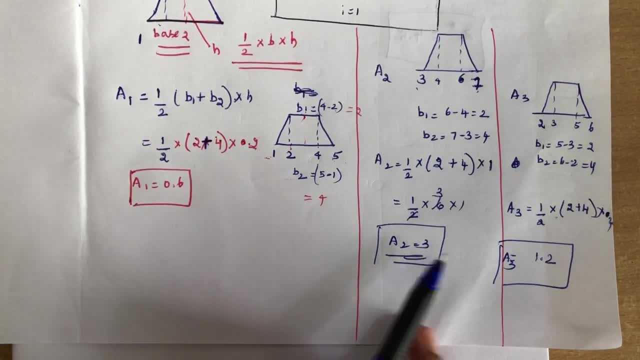 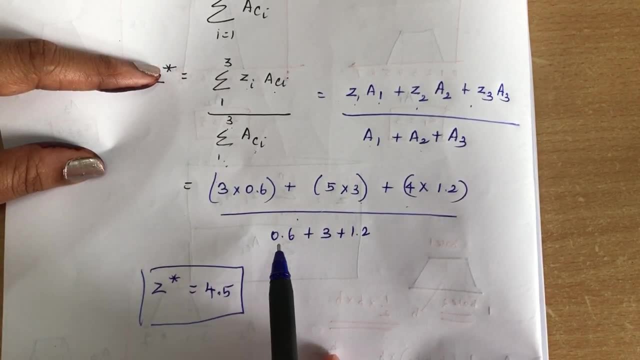 all the areas also 0.6, this is 3 and 0.2.. So when I substitute here, I am getting 3 into 0.6, plus 5 into 3 plus 4 into 1.2, divided by 0.6 plus 3 into 1.2.. So I am getting the. 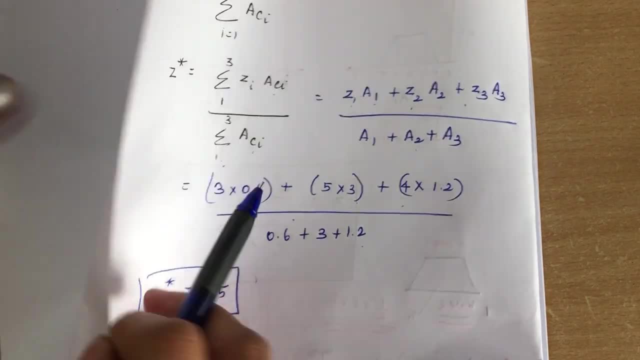 answer to be 4.5.. So using this mean using the center of sum method, the de-facified value, I am getting the answer as 0.6.. So I am getting the answer to be 4.5.. So using 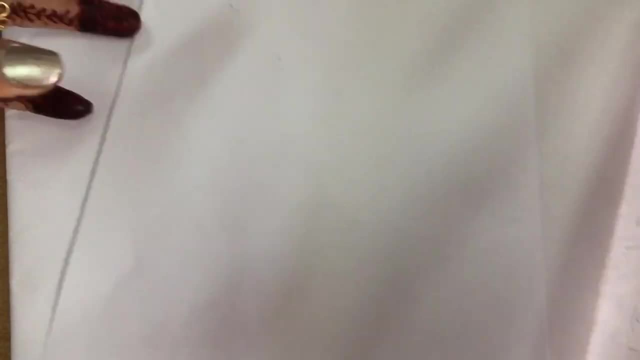 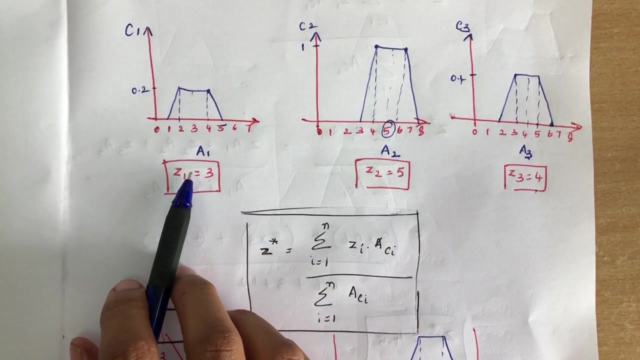 the center of largest area method, I am getting the answer as 4.5 method. okay, This is very simple. So first I need to find out the area bound by all this region and then I need to find out geometrical centers. So by multiplying the geometrical centers into area and taking 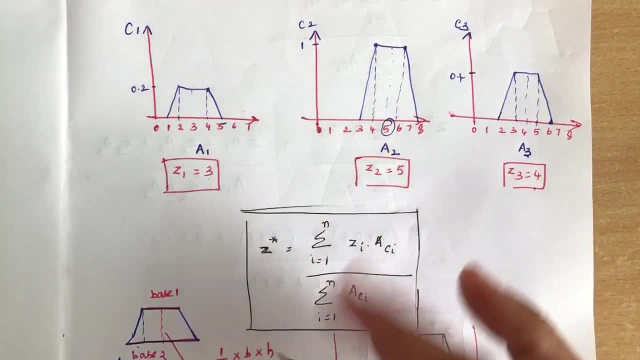 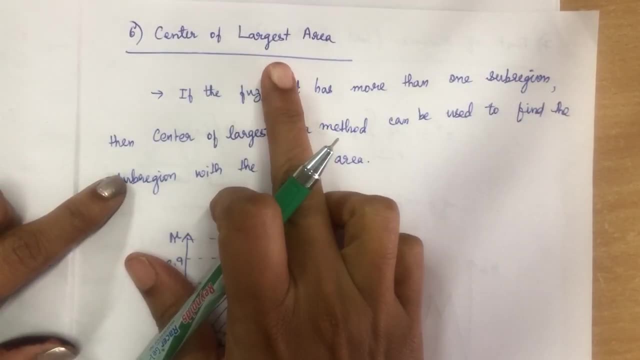 algebraic sum divided by the areas, divided by algebraic summation of areas, you will get your de-facified value. okay, Next method is center of largest area method. So in this method you will be finding out the de-facified value by using, by multiplying the area by 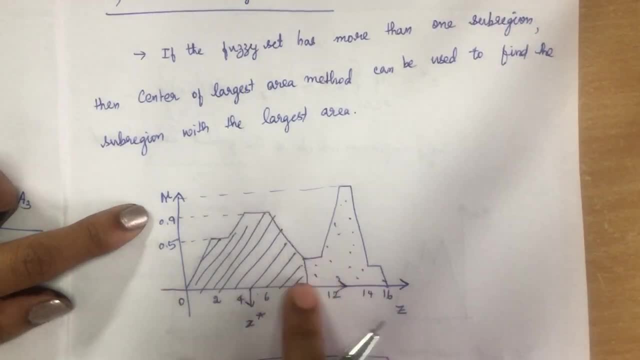 by calculating the largest area. suppose, for example, if you are having two or more regions, so we need to find out the area of every region. so among the region, whichever region is having the largest area, so that will be chosen and we will be finding out the center value so that 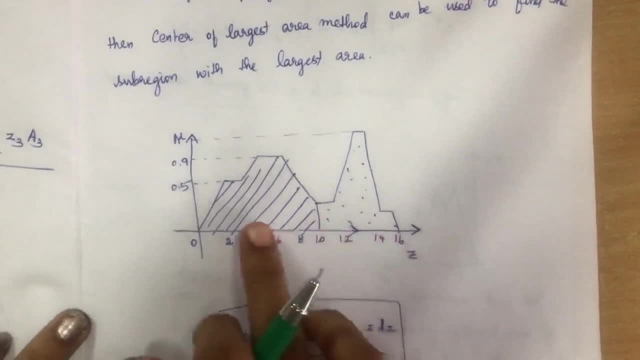 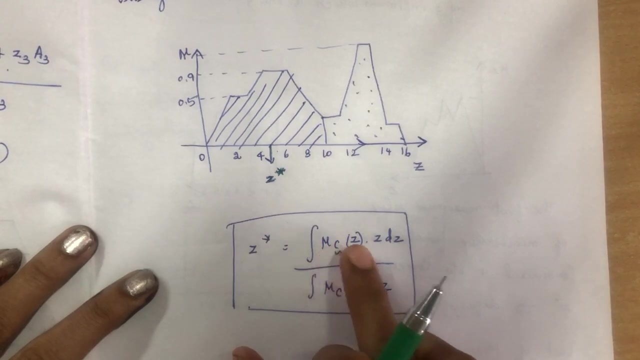 value will give you the de-fuscified value. so among the two regions, this is the largest area and we will find out the center value. this value corresponds to z star. that will give you the de-fuscified value, z star. so z star will be finding the integration of membership value of. 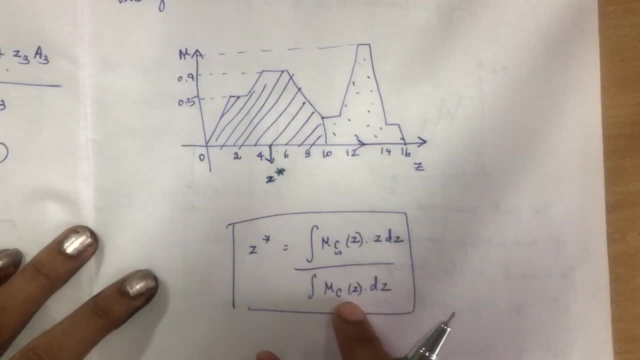 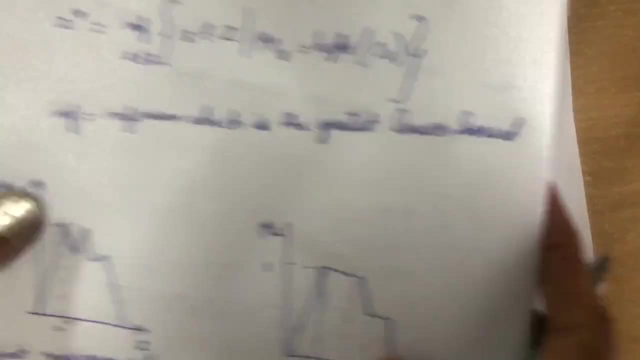 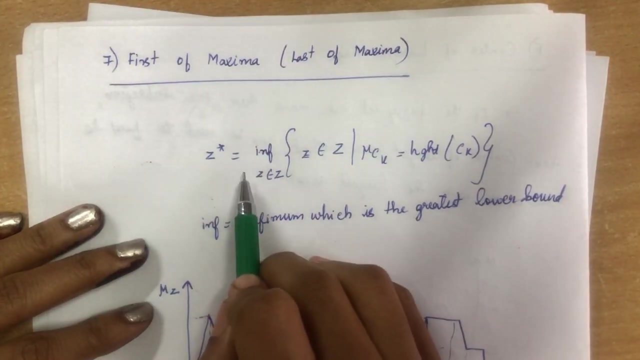 z into z dz divided by integration of membership value of dz. okay, this is how we will find out, by using center of largest area. next one is first of maxima or otherwise last of maxima. so coming to first of maxima. so we will use this formula to find out this first of maxima. so the de-fuscified 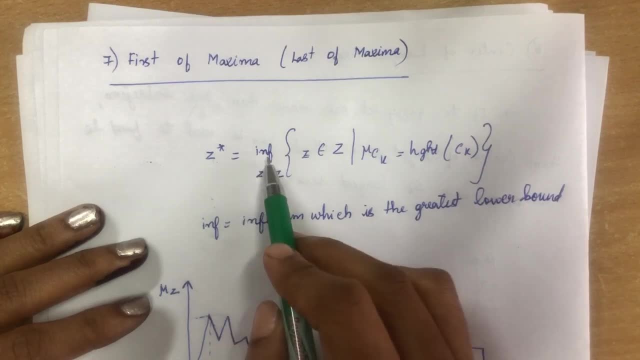 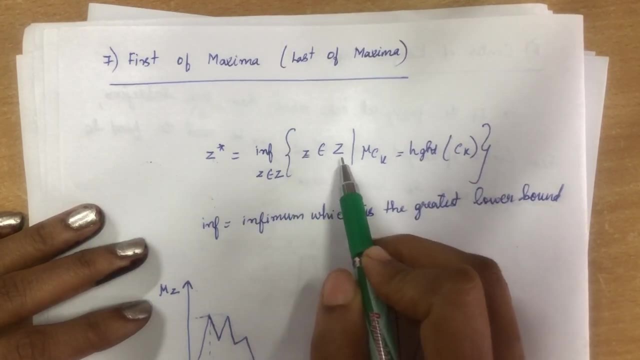 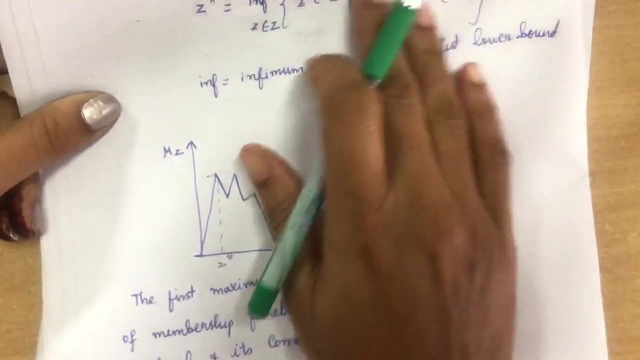 value z star will be will be find out by finding the infimum. infimum is nothing, but it is a greatest lower bound infimum of z that belongs to z, such that membership value of c k will be equal to height of c k. so what do you mean by this? this formula looks very little bit difficult, but when you go for the 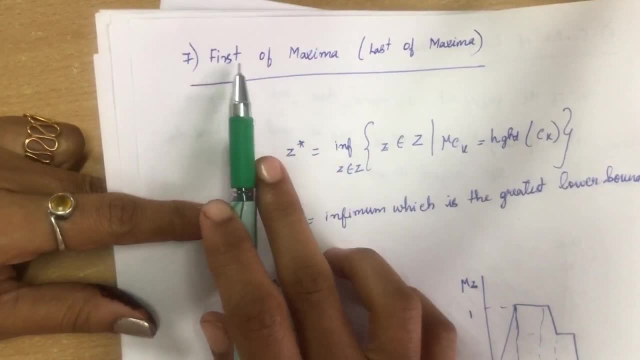 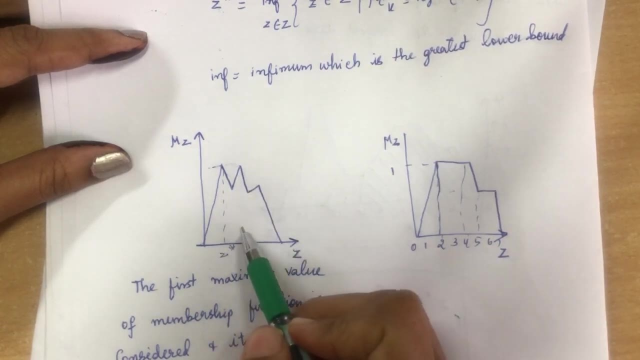 numerical example. it will be very easy. by the name itself it says that it is first of maxima. so if suppose, if you are having three regions which is formed by union of three, first of maxima, c sets, so the first of maxima will be. so here you can see this: the two regions, two points are having 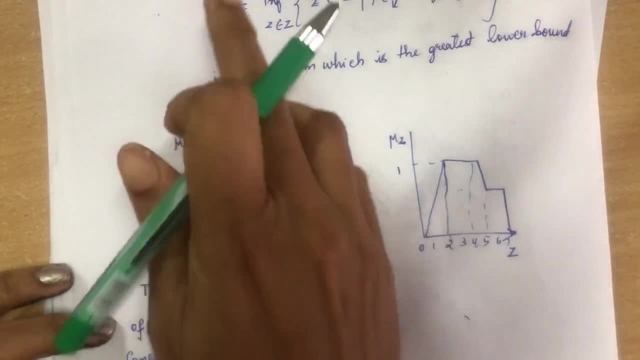 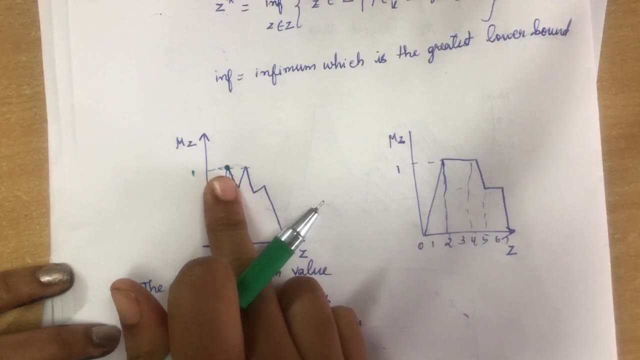 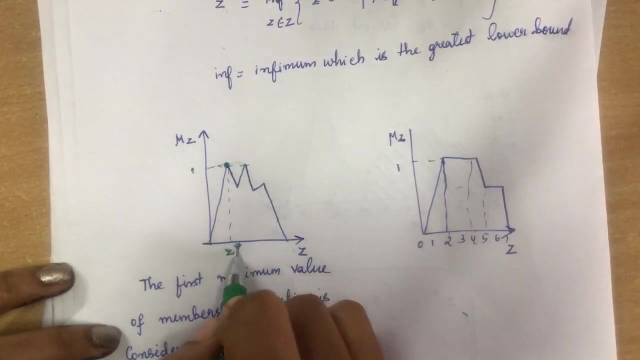 the same membership value called one. but this first of maxima will choose the de-fuscified the. it will choose the, the first maximum value of membership, first maximum value of membership function, that will be the de-fuscified value. that corresponding z star will give you the. 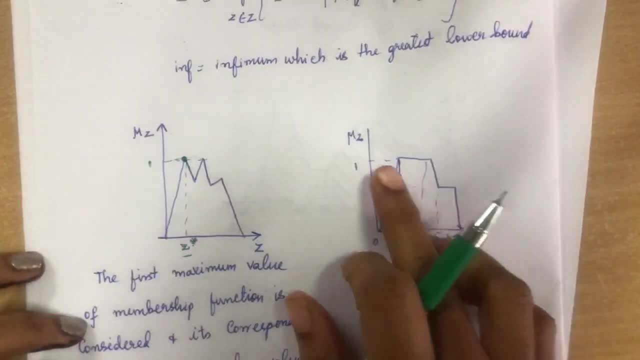 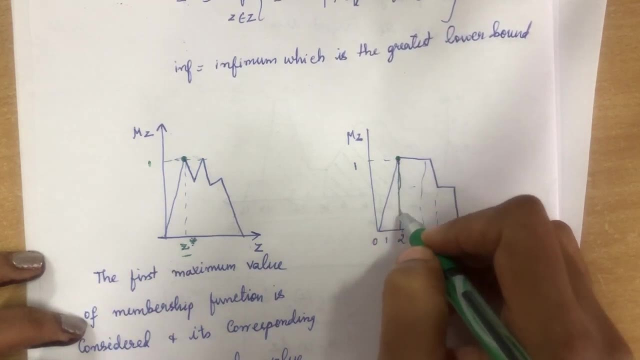 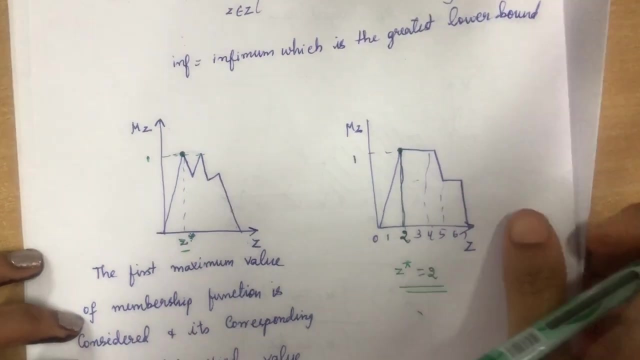 de-fuscified value. this is your first of maxima. so, for example, if you have this particular region, so here the first maximum values, this point and its corresponding z star is two. so z star will be de-fuscified value will be two over here. okay, so now what is last of maxima, last of 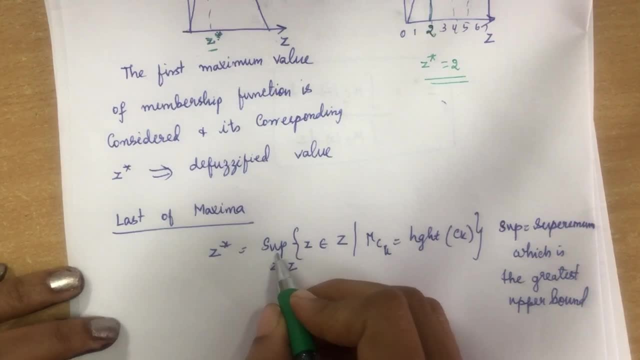 maxima is same, but it is opposite to this: it is. instead of writing infimum, we will write supremum over here. supremum of z that belongs to z, membership value of c? k will be height of c? k. that is supremum, which is the greatest upper bound. 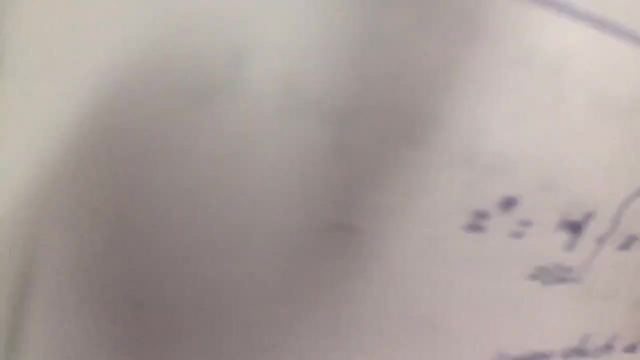 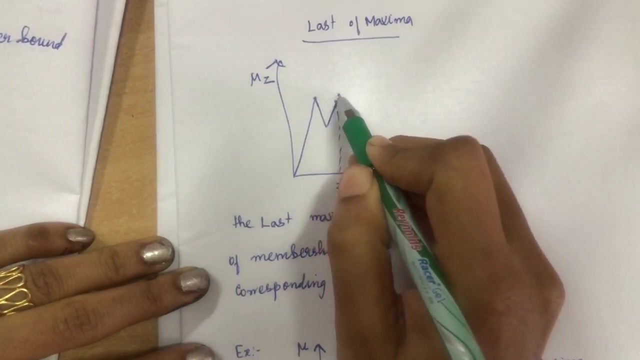 okay. so coming to this diagram, the last of maxima. so here we have this particular fussy set where it is having two points or having the membership value one. so last of maxima will choose the last maximum value of membership function. so here it will not choose this. 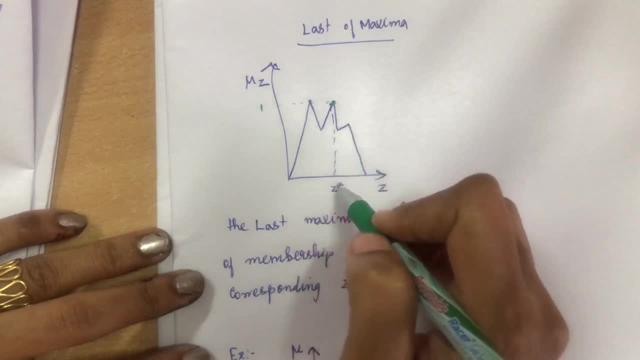 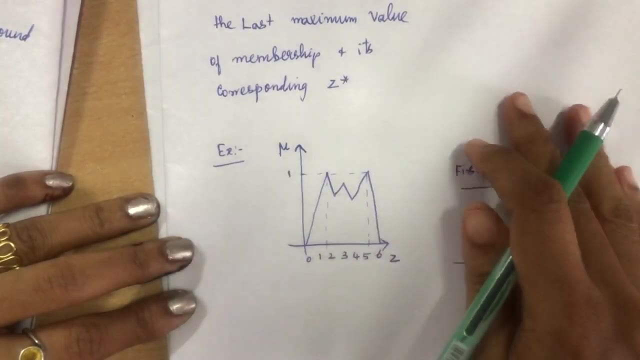 particular point. this will choose this particular point. the corresponding z star will give you your de-fuscified value. okay, so, for example, if you are having this particular membership value region, so what will be the first of maxima? the first of maxima will be so here, this point. so